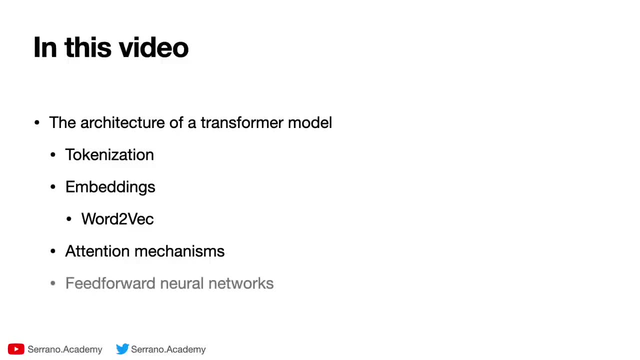 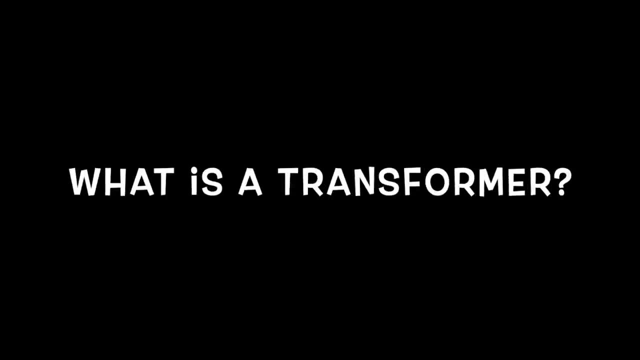 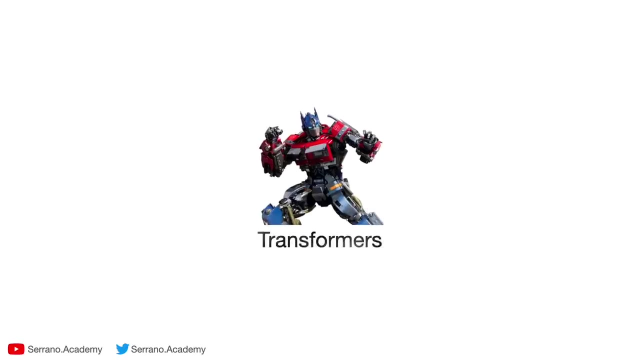 the previous two videos. so I'm just going to tell you the idea here. And finally, I will tell you about feedforward neural networks, which are the main engine of a transformer model. So let's start with the first question: What is a transformer? Well, this is how I imagine a 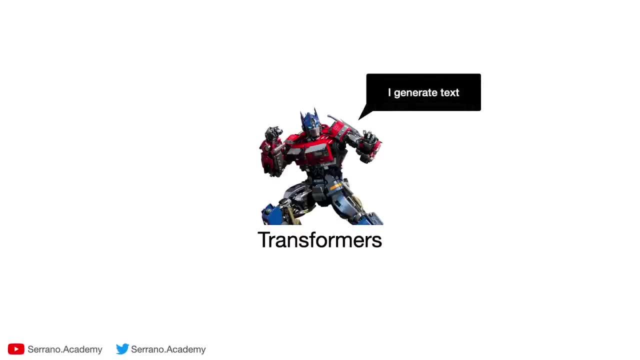 transformer And, as you've seen before, it generates text. Now, how does it generate text? Well, you'll be surprised. It actually does it one word at a time, So you may have seen that it generates really long and elaborate responses. It actually does them one word at a time, So for 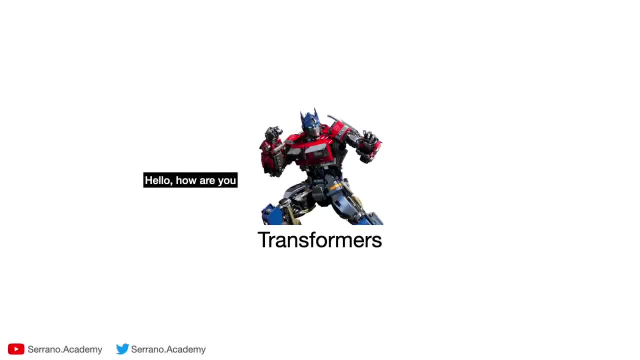 example, if the prompt or the question is hello, how are you Then? it doesn't generate an answer, It only generates the next word that would come here. So what would the next word be here? Well, it can be many things, but perhaps the word doing So. then now you have the sentence hello. 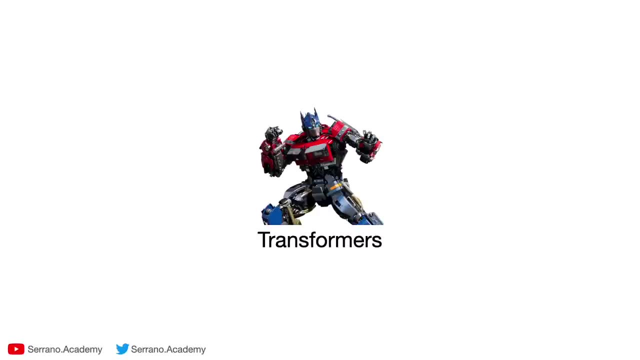 how are you doing? Now you can come up with more complicated prompts like: write a story. Now, the transformer is not going to write a story right away, It's just going to generate the next word. What's the next word after write a story? Well, perhaps it's once, because it's starting the story. 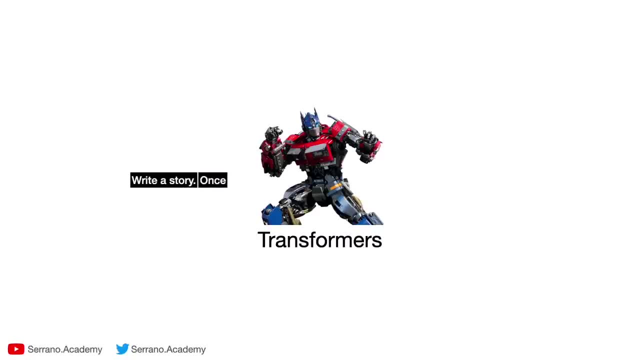 and then it restarts. So now it prompts: write a story once. What's the next word? Well, perhaps it goes. write a story once upon. What's the next word? Well, it's a, and it keeps going. Write a story once upon. a generates the word time, etc. etc. And if it does this many times, it will. 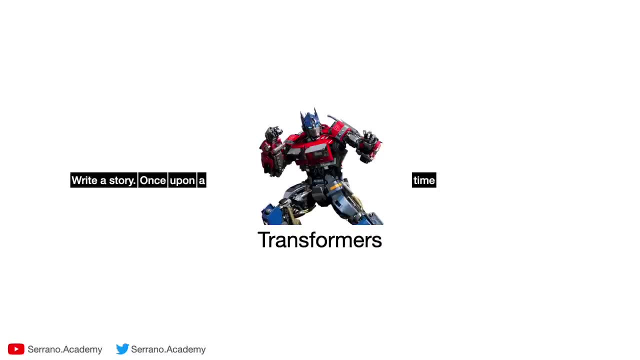 actually generate a story Now. you may have been as surprised as I was. I first thought it would generate the entire response right away, or maybe it would come up with an idea and start elaborating on it. But no, it actually just goes one word at a time Now. in order to generate one word at a time, 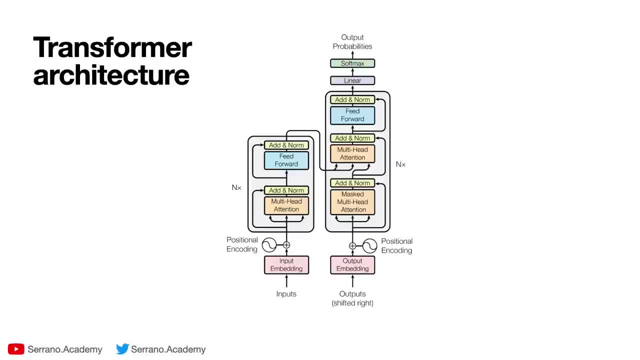 here in language. it actually needs a lot of parts. So this is the architecture of a transformer. It looks complicated with a bunch of things called input, embedding, multi head, attention, feed forward, etc. But in this video I will break down all of these blocks one by one. Actually, 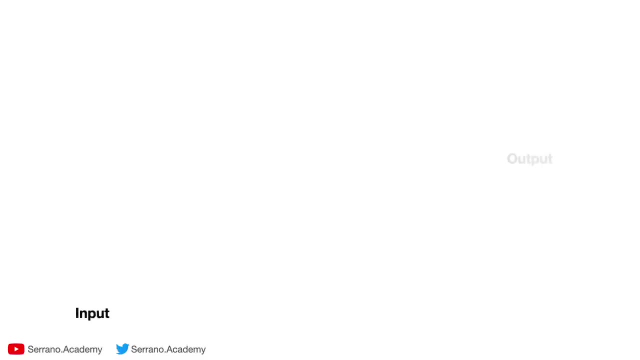 the way I like to see it is more like this: you have an input and an output, And let's say the input is write a story And the output has to be probably the word once. But what happens here? well, first it goes to a step called tokenization, then a step called embedding. 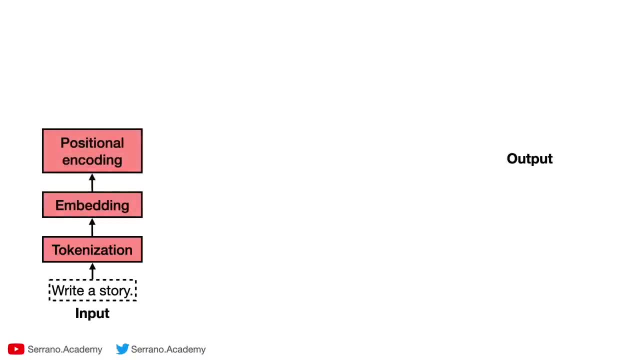 then a step called positional encoding. This is more of a pre processing. then it goes through the main engine, which is a series of transformer blocks, And these all have something called attention, which you saw in the first two videos, and feed forward, which is a neural network. 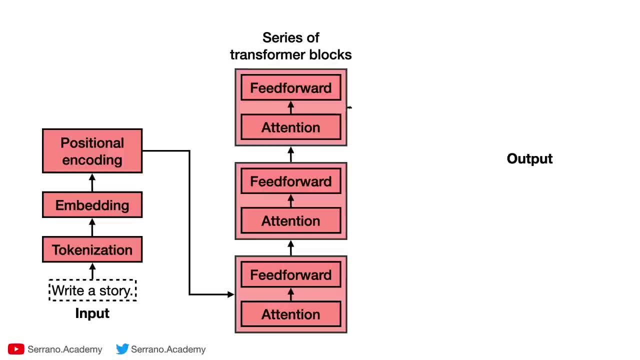 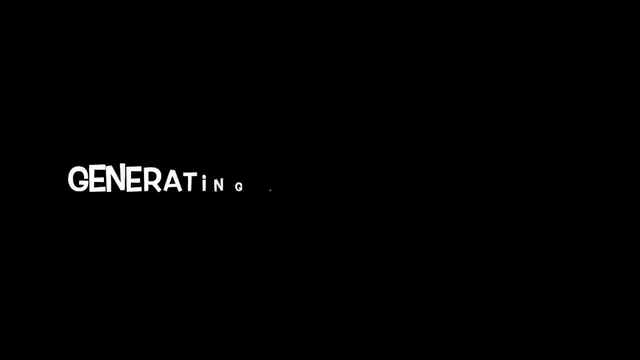 there can be many blocks here, And then at the end, there is a block called a softmax, And out max comes the answer, which in this case, would be the word once. So fasten your seatbelts, Because in this video, I'm going to tell you about all these parts. Now, before we get to the architecture, 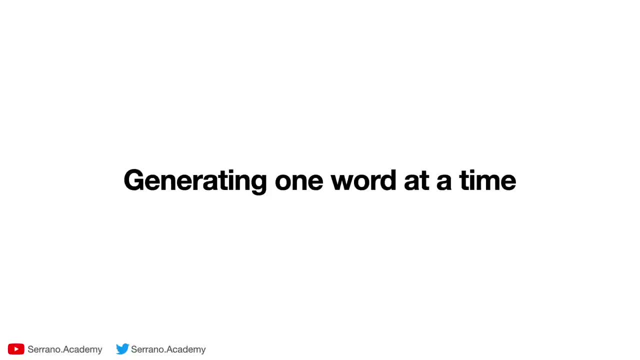 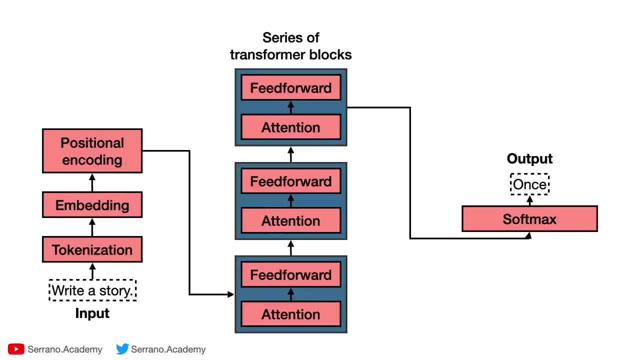 of a transformer. let's take a look at this concept of generating sentences one word at a time. Recall that the architecture of transformer is this one: where the main engine is in the middle is a series of transform blocks, in particular the feed forward part. 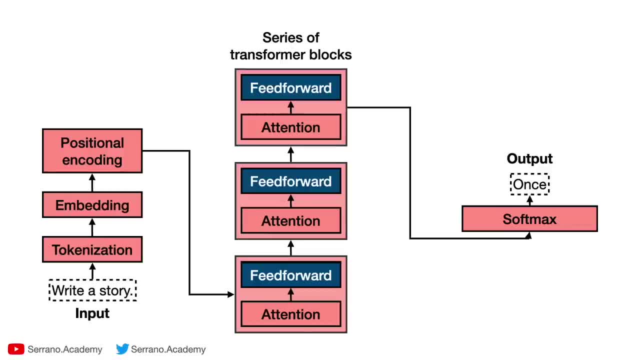 It's a neural network that tries to find the next word in a sentence, And all the other blocks are there to help this neural network work as best as possible. But this concept of generating the next word in a sentence is something that has been around for a while. Can you think of a time? 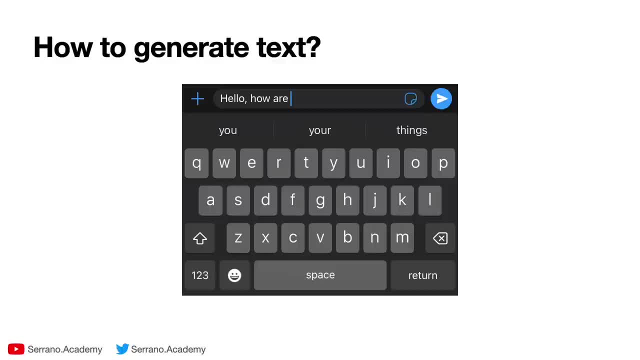 where you have used it. Well, if you have texted anybody, you may have noticed that the texting apps have these suggestions. You say the sentence Hello, how are? and it generates three suggestions: you, your and things. And let's say you pick the word your. that means that your. 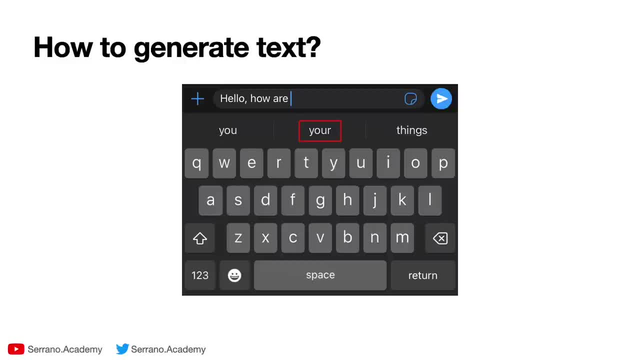 sentence will be: Hello, how are your? and then, after you type your or you press the middle button, then three more suggestions will appear based on the sentence you've given it. Now let's think about the following. Let's say that you have 10 minutes and you are given the task of creating 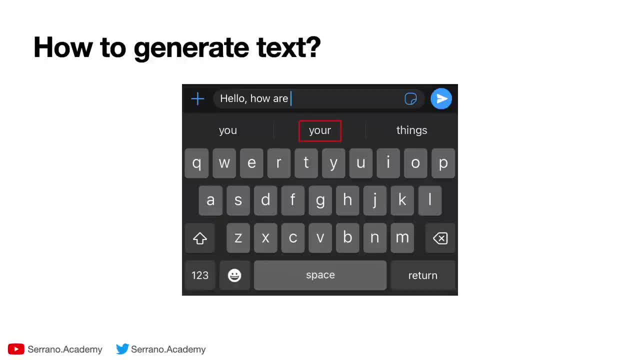 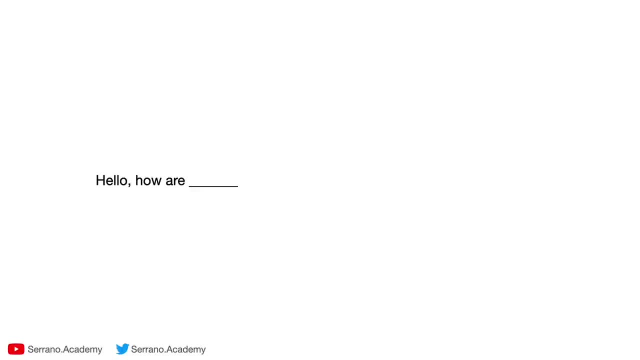 a model that suggests the next word in a sentence. What would you do if you only have 10 minutes? Well, here's a simple solution. Let's say that you pick the last word, the word are, and you think what is the most common word after the word are. Well, if you have a large data set of sentences, 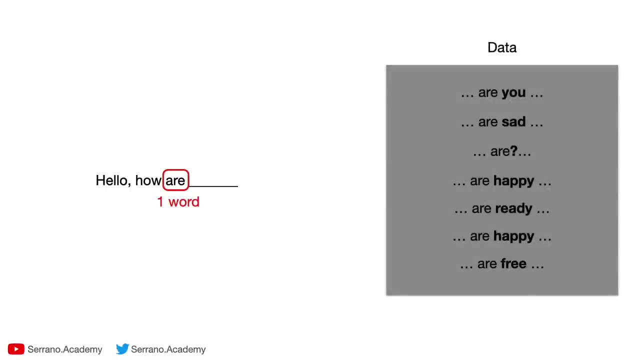 you can just look at all the instances of are and then pick the most common word after, in which case here is happy, And so you suggest the word happy. Obviously that doesn't work very well, But at least it suggests words that could be sensible. This has a name, is called a. 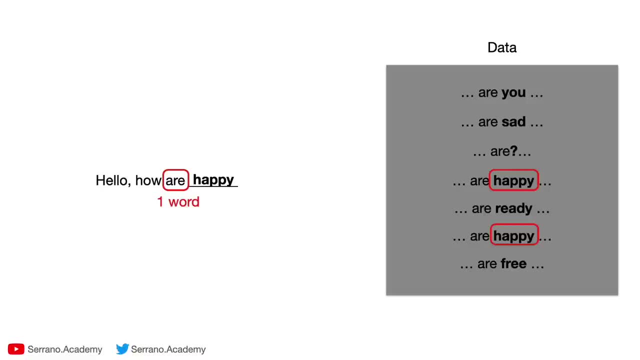 one gram. Now can you think of how to make it more complicated? Well, let's look at a three gram. A three gram is when you take the last three words, hello- how are? and then think of what's the most common word that comes after. So you look at all the instances of hello. how are in your data? 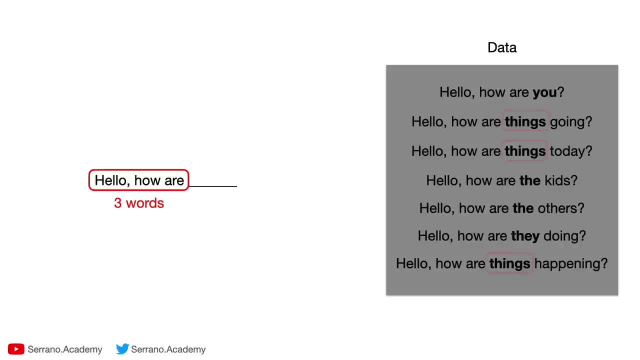 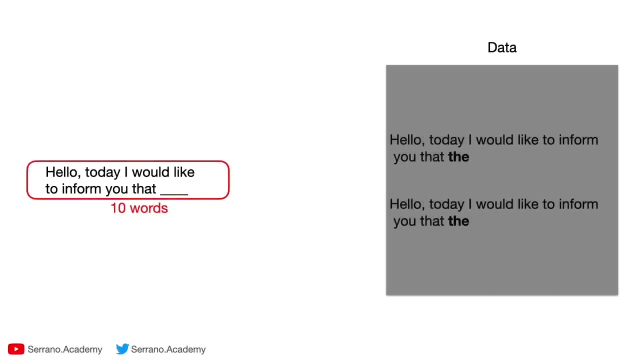 set of sentences And let's say: the next most common word is things. So you suggest the word things. Now, how can we make this even more powerful? Well, let's do a 10 gram. You pick the word things- I would like to inform you that- and then find that in your data set. And let's say: 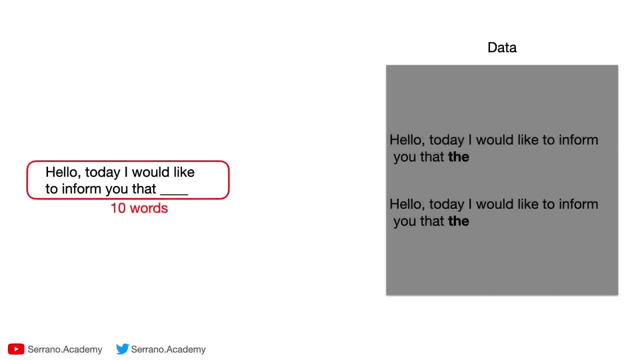 that it only appears two times, But both of them are followed by the word the. so you suggest the word that. now, what's the small problem here? Well, the more words we pick, the more educated the guest is. but also, the more words we pick, the less likely that that sentence could appear before. 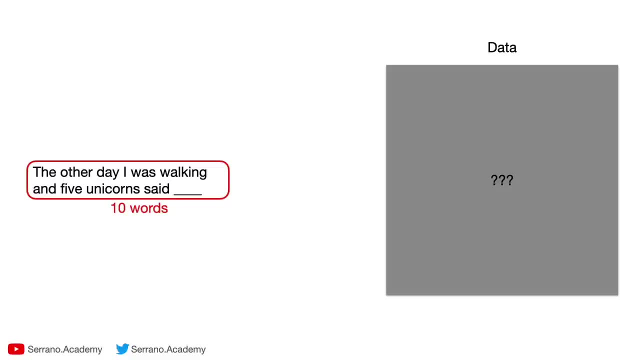 if I take a sentence like the other day I was walking in five unicorn said: well, that sentence may never appear, because it could have been the first time somebody says this sentence. So you can't rely on just looking at words that appear before, because it may be that they've never. 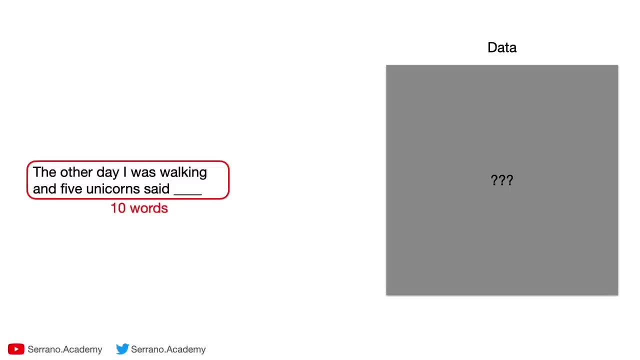 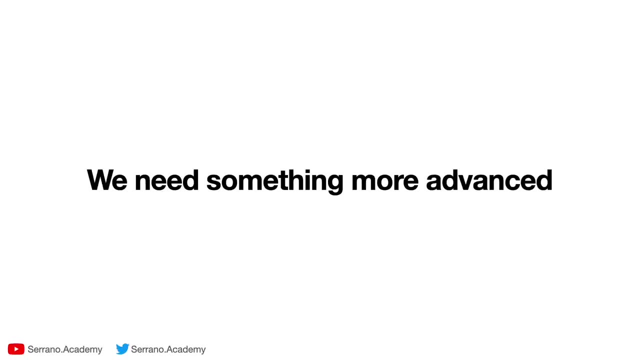 been said before, However, this method sometimes is used, and it's called the n-gram method. n is the number of words you're looking at, So this one would be a 10-gram, But it looks like we need something more advanced. So what can we do? Well, something that's been used for many years in order 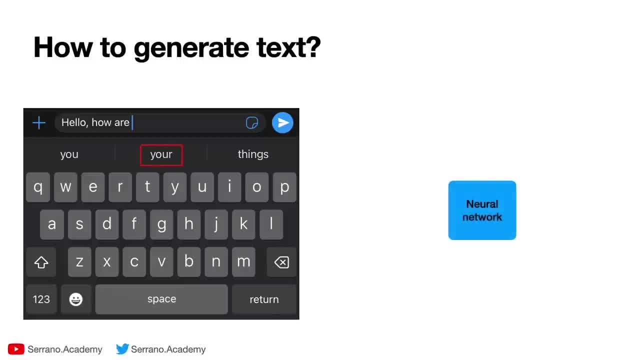 to suggest. the next word is something called a neural network. So in a neural network you input the sentence hello, how are, and it outputs the word you are. Now I'm not going to go into detail on what a neural network is. I will go into some detail. But if you want to really learn what neural 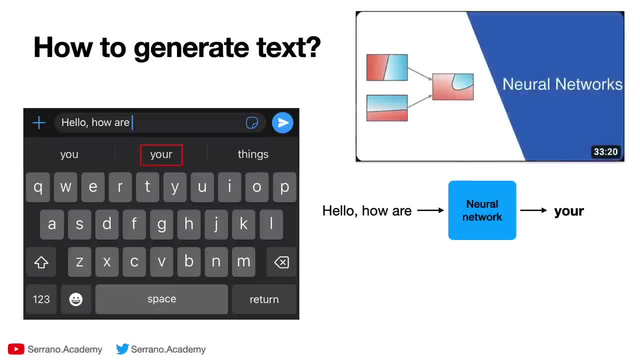 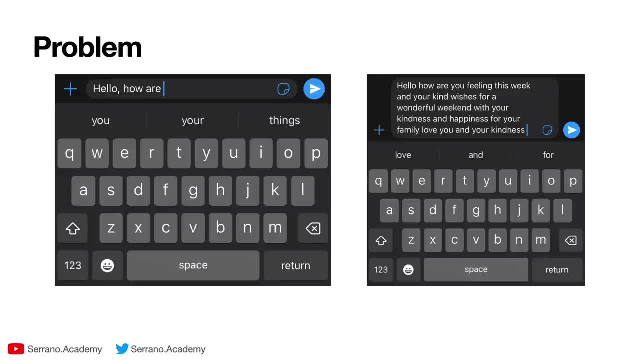 networks are and how they work. check out this other video on my channel called neural networks. The link is on the comments. However, up until transformer, these things didn't work that well. I don't know if you've ever tried to actually write a text by pressing the suggestion in the 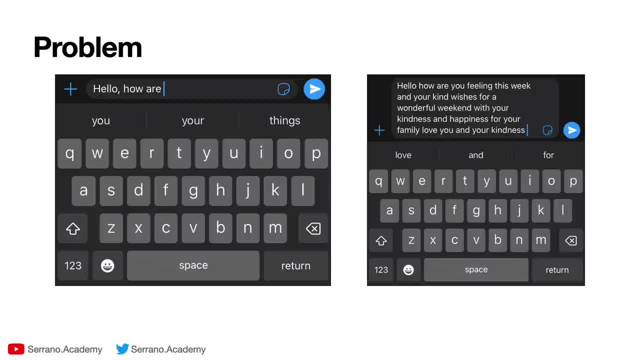 middle. I tried doing it And it gave me the sentence: Hello, how are you feeling this week? and your kind wishes for a wonderful weekend with your kindness and happiness for your family. love you and your kindness. That makes absolutely no sense, But if you look at every three or four consecutive words it makes. 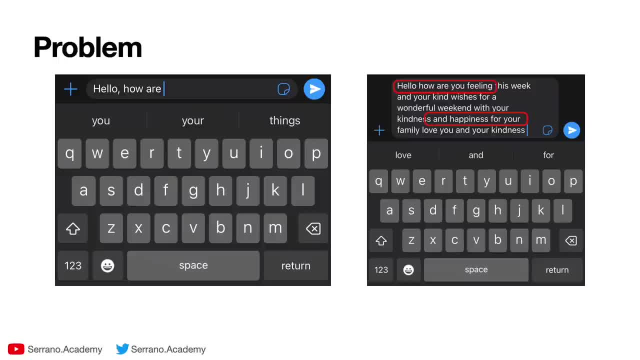 sense. Hello, how are you feeling? and happiness for your, etc. etc. Because this neural network is trained to remember a few words at a time and to build short sentences, not to build long text. And to build long text, we need a transformer. 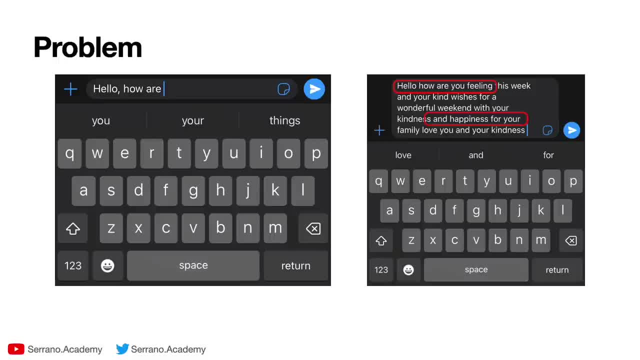 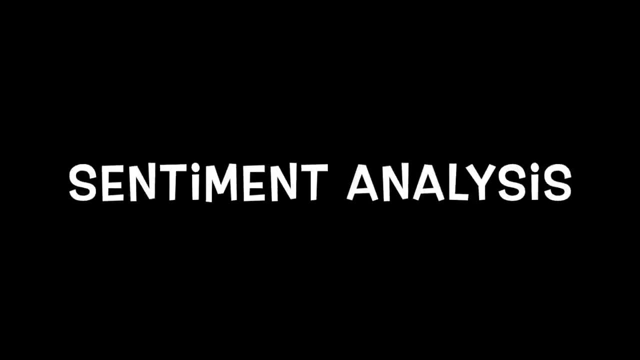 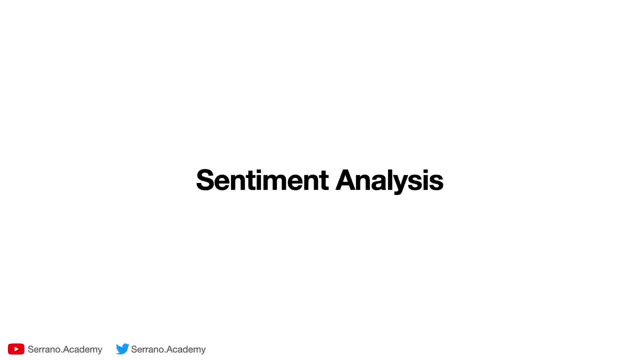 But first let's take a little look at how these neural networks work, because they are the key to understanding a transformer model. So before we get into how neural networks generate the next word in a sentence, let's look at a simpler example, which is called. 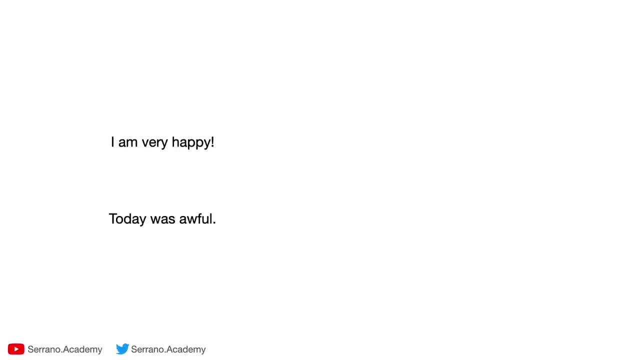 sentiment analysis. Sentiment analysis has been around for a while and it's one of the quintessential problems in natural language processing, And it basically consists on building a model that is able to tell if a sentence is happy or sad. For example, the sentence I am very happy is a happy. 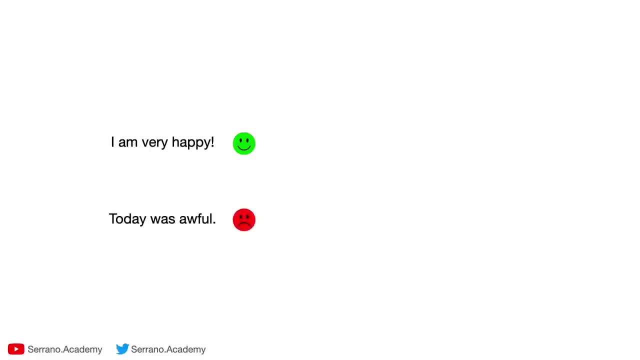 sentence, And the sentence today was awful is a sad sentence, And the idea is that you can use a data set that has been labeled. So you have a lot of sentences and you have the information on if these sentences are happy or sad And based on that data, you can build a 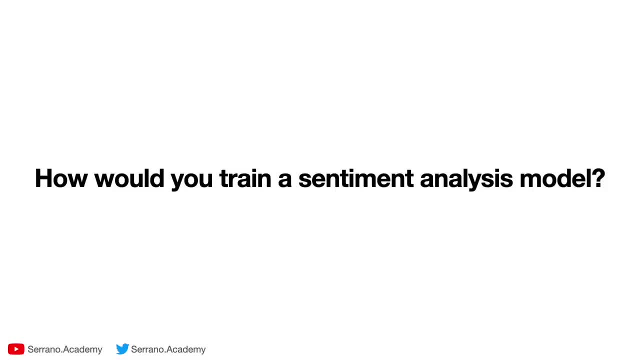 model that is able to tell if a new sentence is happy or sad. Now the question is: how would you train a sentiment analysis model? so i'd love for you to pause the video and actually give it a thought, if you haven't seen it before. 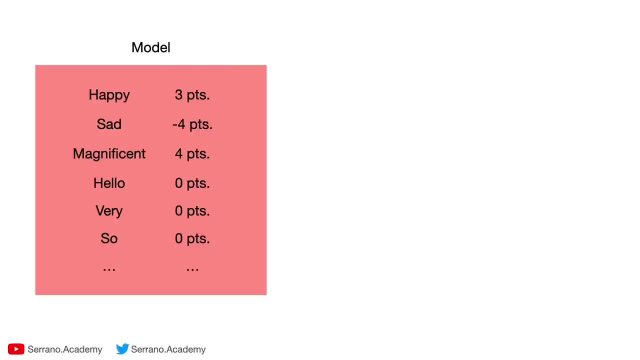 here is a way to do it. a way to do it is actually to have a set of points, a score for each one of the words. so happy words will have positive points, sad words will have negative points and very happy words, like magnificent, will have more points than okay, happy words like happy and for the 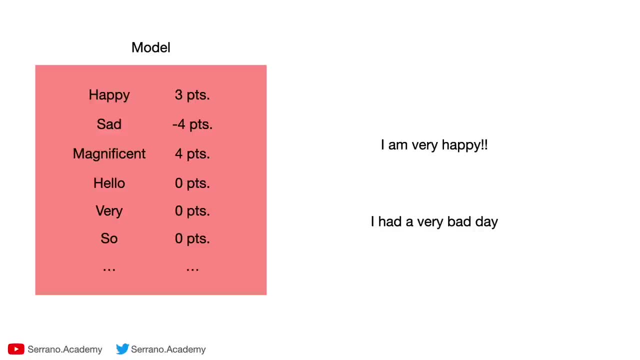 rest of words that are neutral, they will have zero points. so if i were to have such a model, if i were to have such scores, then i can easily tell if a sentence is happy or sad, for example, the sentence i am very happy. well, what's the total score of the sentence? the words i am and. 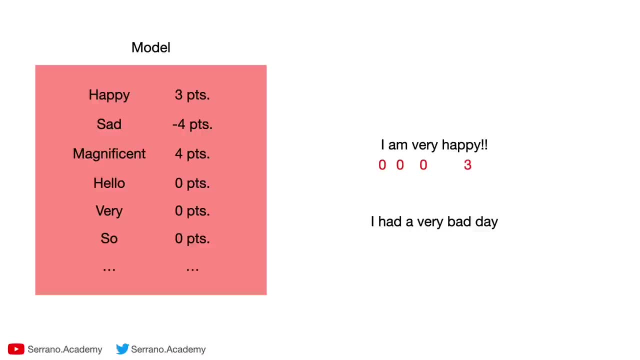 very are neutral, so they have zero points, and the word happy has three points. so when i add them i get three points and if the score is positive, i conclude that the sentence is happy. now for the sentence i had a very bad day. the words i had a very and day are all neutral, so they have 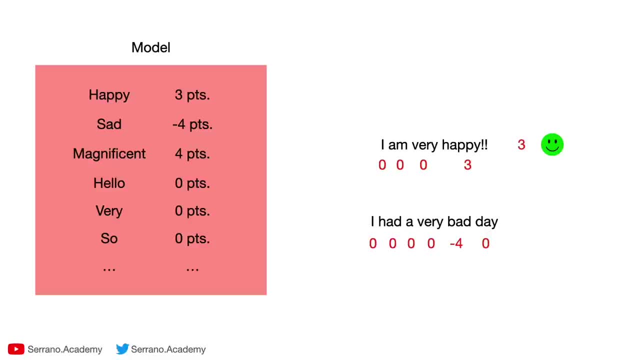 zero points and the word bad has minus four points because it's a sad word and therefore when i add them, i get minus four, which means that the sentence was sad. now, the idea is that a good sentiment analysis model will have points for every single word, and if you 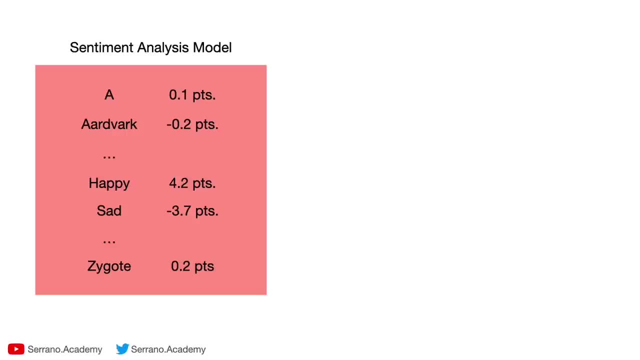 are able to score every word. i haven't told you yet how to score them, but if you are able to score them, then you have a sentiment analysis model and this looks like this. i'm going to put all the words on the left, each one with a red node and a node on the right. 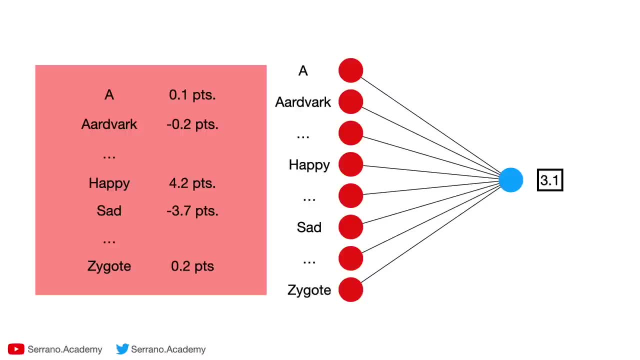 right and then connect them all with an edge. and on the edges i'm going to put the scores that we found so: happy is 4.2, for example, sad is minus 3.7 and all the other ones. and now when i have a sentence like i am happy, then i simply locate the words i am and happy, i put ones on them. 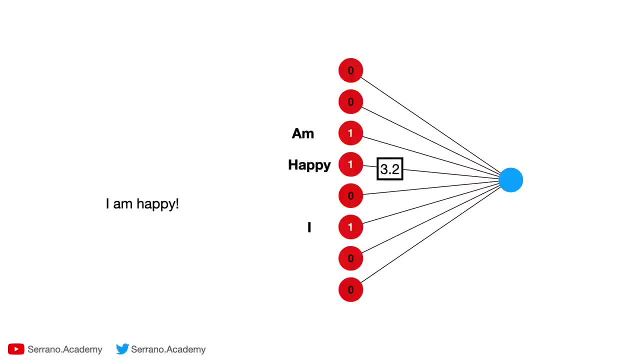 and then i multiply these ones by the scores in the edges. i actually multiply every score here by the score on the edges, but most of them are zero, except for the words in the sentence, and then i add them. so when i add them i get 3.2 plus 0.1 minus 0.2, and that's 3.1. so i conclude that this sentence is happy. 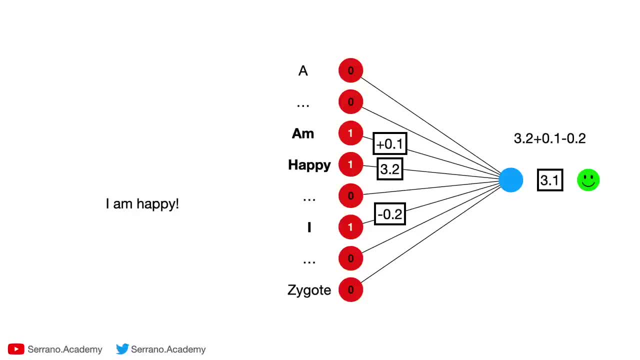 this is called a perceptron, and if you've seen perceptrons before, you may have noticed that i didn't talk about the bias unit. there is also a bias unit. there is a constant that we add to all these sentences and it takes into account empty sentences. if empty sentences are happy or sad, 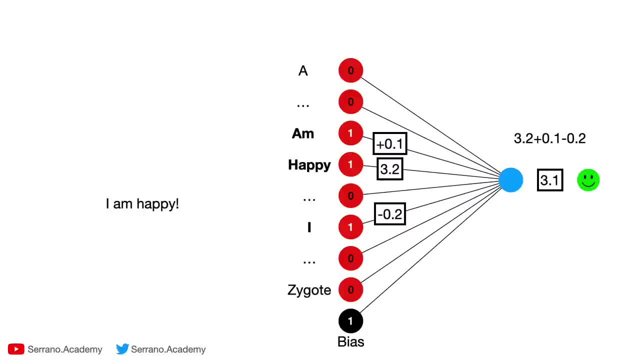 then only the bias can tell us that. but, as i said, this video is not about neural networks per se. if you want to know more about perceptrons, the bias unit and these scores and in particular how they work for sentiment analysis, check out this video on my channel, called logistic regression. this 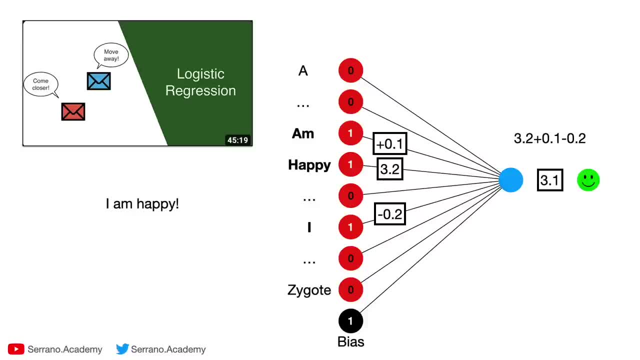 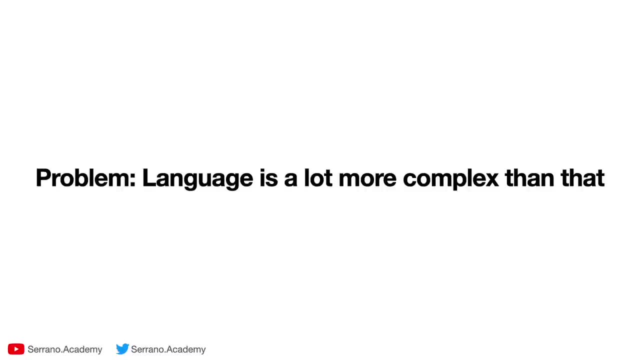 video will also tell you how to train a neural network, which is how to find these very good scores for each one of the words. now the problem is that this is not going to work all the time because language is a lot of work, and it's not going to work all the time because language is a 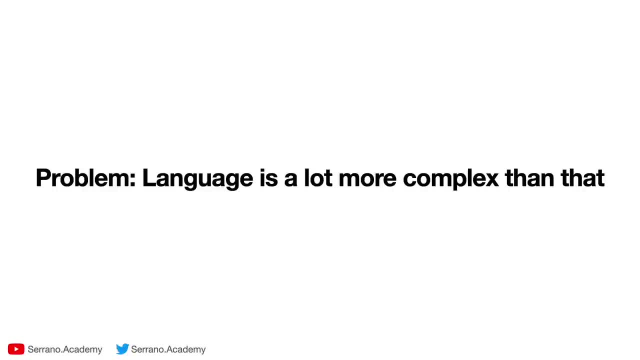 lot more complex than that. if we could just understand language by adding a number to each word and then we know if sentences are happy or sad or they're talking about different topics, then language would be very simple. but it's not, so we need something more complicated than that. 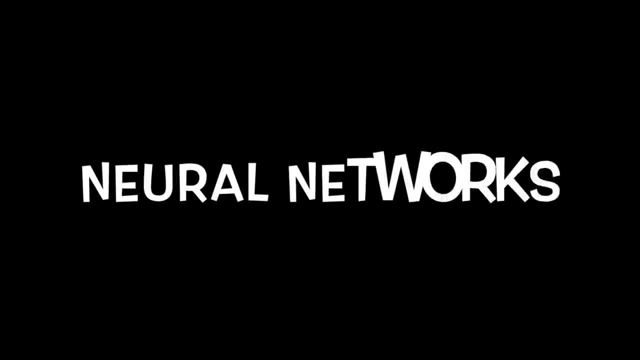 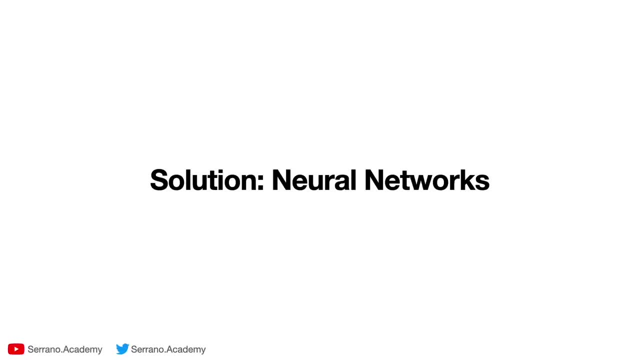 and that's when we jump to neural networks. now let me show you what a neural network is and how it can help us with the sentiment analysis problem. so here is the graphical representation that i showed you before of a very simple sentiment analysis model, and notice that it looks a lot like a neuron, like 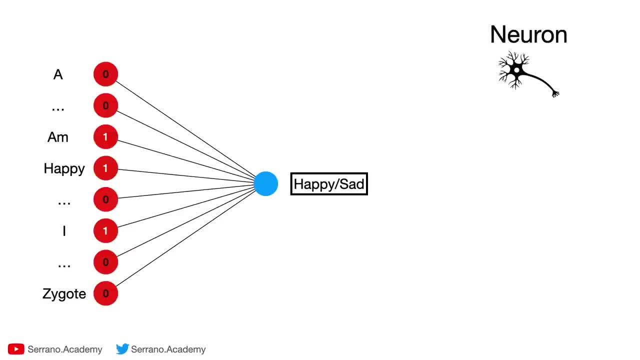 a brain cell because it has a lot of inputs. in this case, each word is a potential input and one output, which is if the sentence is happy or sad. this is called a perceptron and it's the basis of neural networks, and the output is one if it's happy and zero if it's sad. now, just like brains. 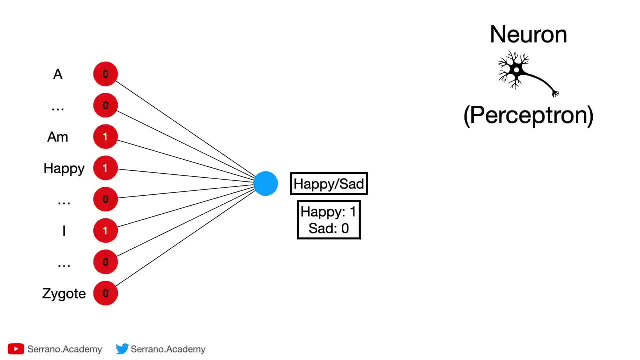 they don't have just one neuron, they have lots and lots of neurons. well, a neural network is formed by many, many, many of these neurons connected in a very strategic way. now i'm going to tell you the mental picture i have of neural networks. when i think of a concept like happiness, it's pretty. 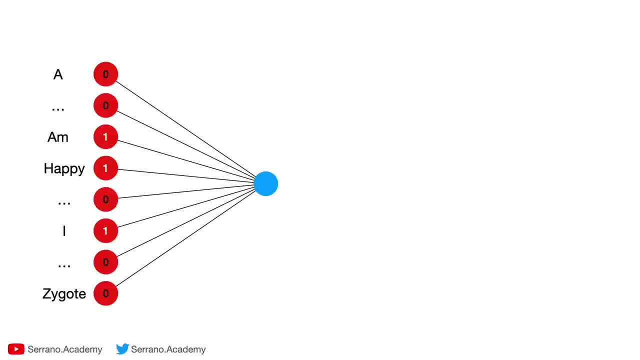 complex. it can't just be determined by having words or not having these words in a sentence. but maybe there are simpler concepts, and maybe one of them could be: if you're talking about family, let's say for the sake of argument that that is a concept that is slightly easier to model with a 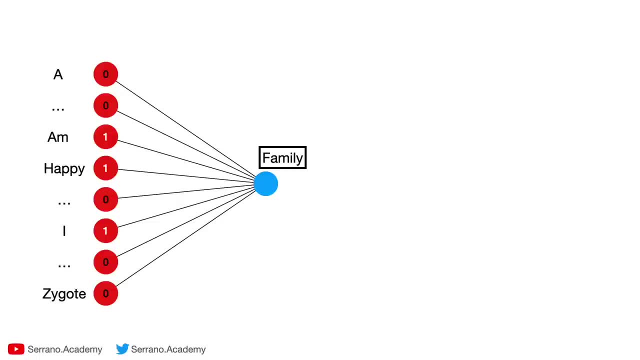 perceptron like this, and maybe there are simpler concepts, but i'm going to tell you the mental picture i have of a neural network. there are some other simple topics that are easy to model, like this: let's say, if you are talking about free time or not. that's a simple concept that can be, let's say, modeled by a perceptron and another. 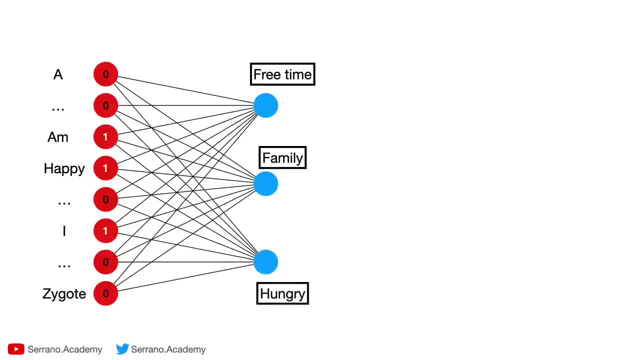 one is if you are hungry or not. and so we have three perceptrons, and each one of them now doesn't tell us if we're happy or sad, but it tells us if we're talking about free time, if we're talking about family and if we're talking about being hungry. and let's just say again, for the sake of 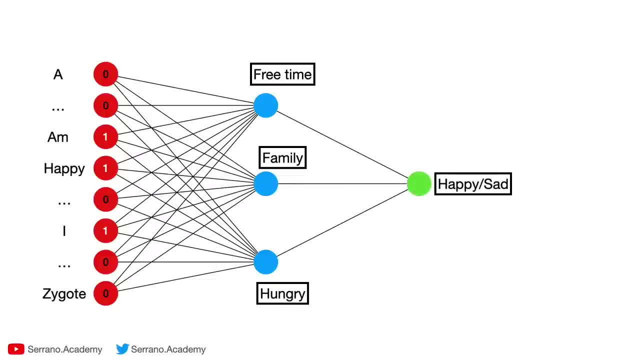 argument that these three determine if we're happy or sad. so if we have free time, if we are happy with it and if we're not hungry, then let's say that determines if we're happy or sad. and we're going to put weights here and the weights can be positive or negative. so, for example, we have a two for free. 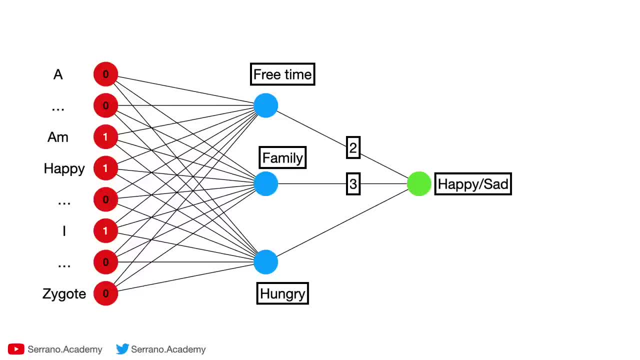 time, because the more free time you have, the happier you are. let's say you have a three for family, because if you have your family then you're happy. and let's say we have a minus two for hungry, because if you're hungry maybe that affects your happiness. so what we have here is a small 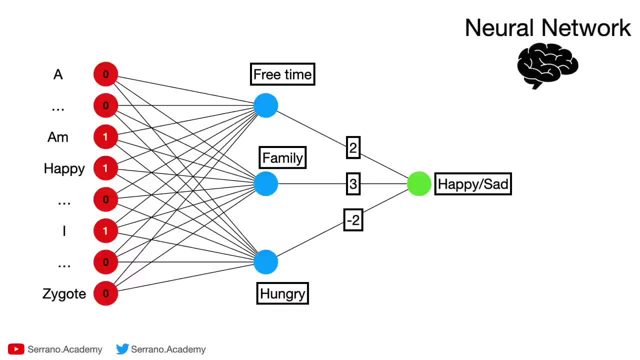 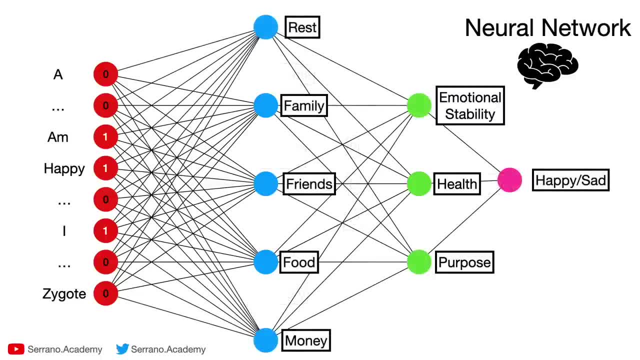 we need more notes like rest, family, friends, food, money, and maybe those don't determine happiness, but they determine other slightly more complex things such as emotional stability, health and purpose, and maybe those three actually determine if you're happy or sad. or maybe there's hundreds of these and they may not be easily labeled for us, but maybe the computer knows. and in the first, 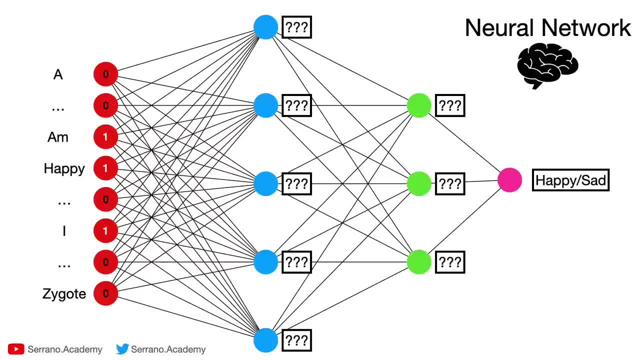 layer you have some simple concepts, then in the next one you have more concepts, and then in the next one you have more complicated concepts, and so on and so on, and you could have tens of these layers or hundreds, and, as you may imagine, if we have a neural network big enough, we may have a 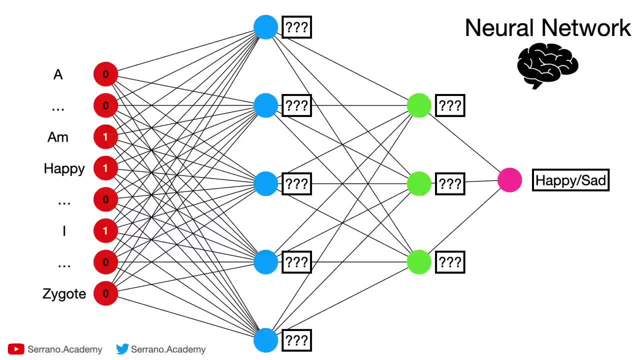 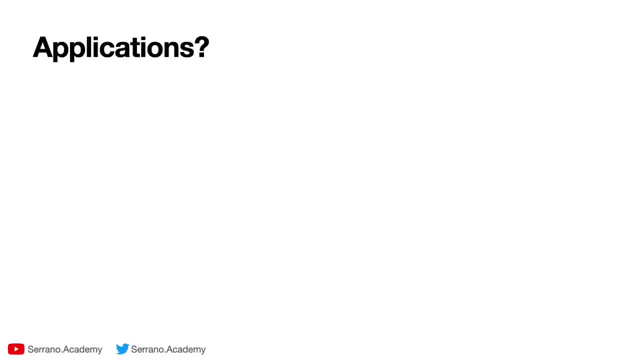 much more accurate way to tell if a sentence is happy or sad. so this is the mental image that i have of a neural network. now these can have many applications. can you help me think of some applications of neural networks? one can be customer support, because you can take a chat with a. 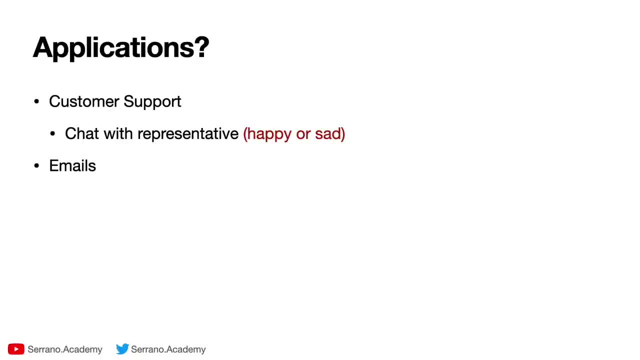 representative and determine if it was happy or sad. you can also use it for emails. you can use it for spam detection. let's say that you train a neural network to tell you if the email is spam or not spam. however, notice that these two examples have two outputs: happy or sad, or spam or not spam. 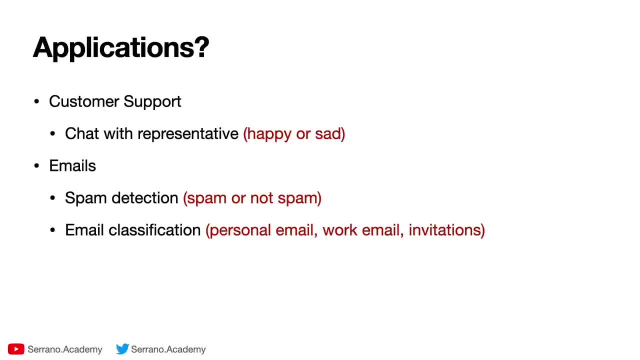 you could actually have a neural network that works for more than two output. for example, email classification. you can classify your email into three: personal email, work email and invitations, or even more so, this opens a new door. now let's think of an extreme case where there's not two or three. 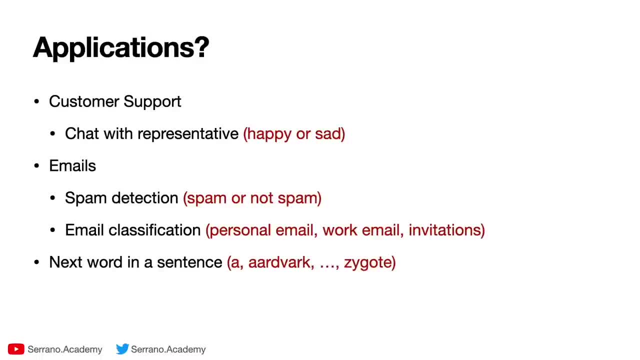 inputs, but there's lots of them. how many of them? as many as words. so i can think of a neural network where the input is a sentence given by a bunch of words and the output is one word out of all the words that exist, and that is a neural network that can predict the next word at a sentence. now, before. 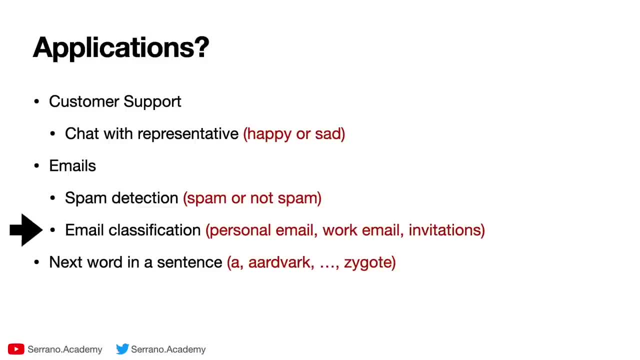 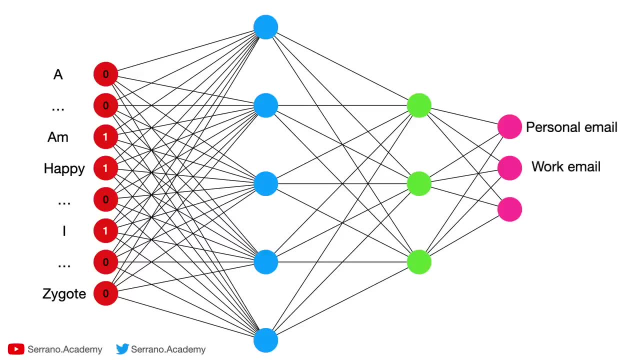 we get to that. let's look at how the architecture would look. so let's look at email classification. here's a neural network that could tell you if your email is spam or not, spam or not spam or not spam, or personal work related, or an invitation. notice that it doesn't have one output. it has three outputs. 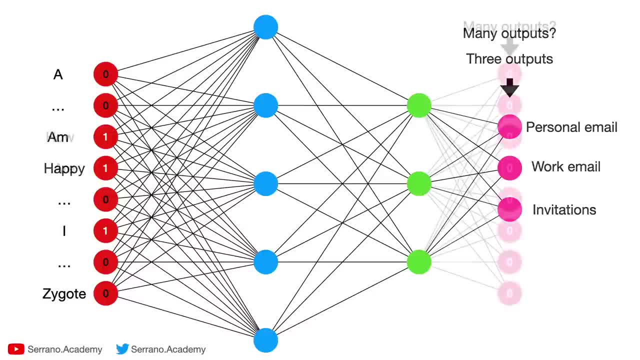 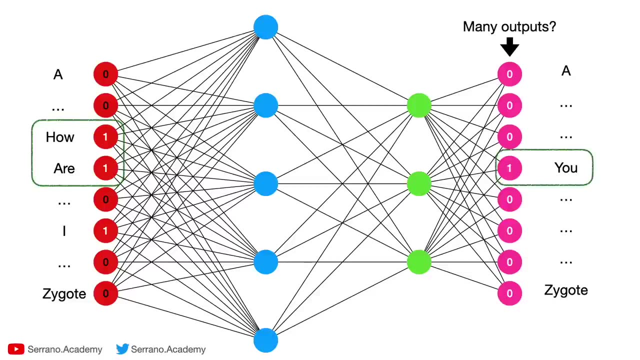 and i can think of many more outputs. i can think of all these outputs up to here, which are as many as the words that are inputted. so in this neural network, the first layer and the last layer have the same size and when you input a sentence like how are, it will output a word which is, for example, 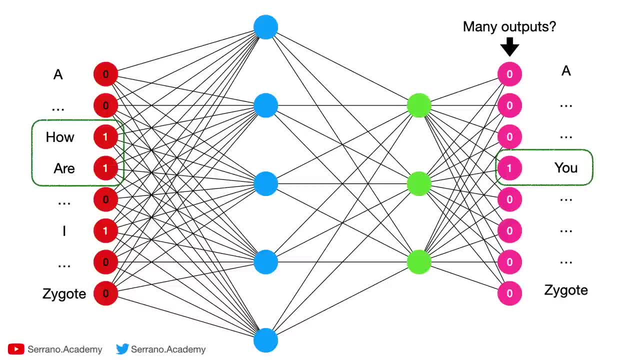 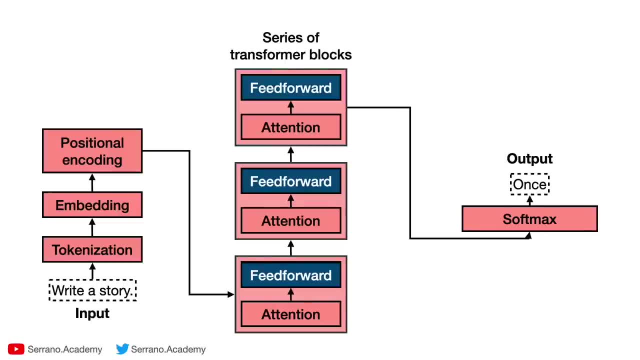 you. so this is a neural network that can predict the next word at a sentence and is very similar to the neural network that appears in the transformer. of course, the neural network- the transformer- is bigger, has more structure, is more complicated, but at the end of the day, it's a big, big, huge neural network that tells the next word of a sentence. however, 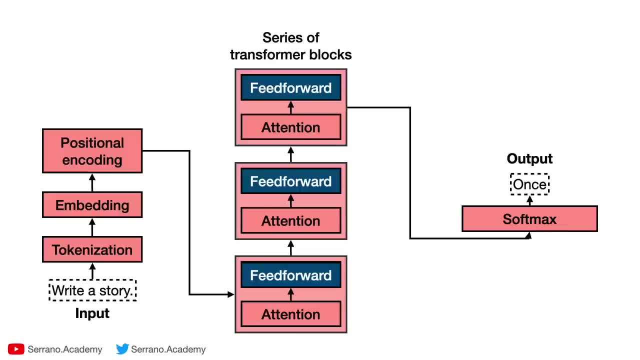 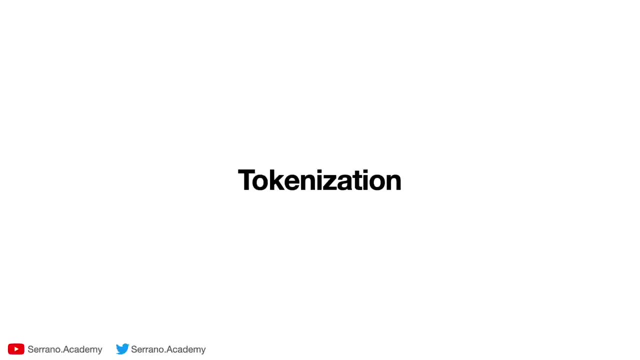 as i said before, just a neural network doesn't do the job. a transformer needs all these other blocks to help it work so well. so now we're ready to go into all these blocks. so the first one of the blocks in a transformer is tokenization, and it goes right after you input. 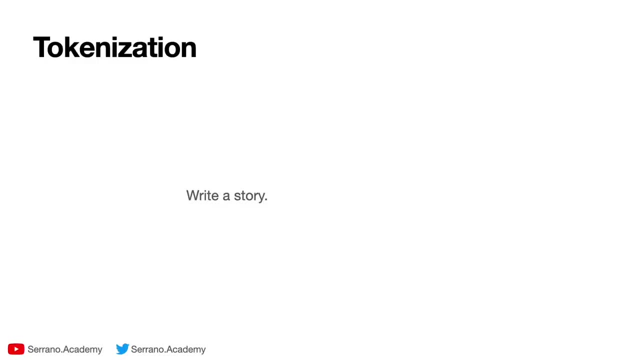 the text and tokenization pretty much breaks everything into units. for the most part each unit is a word. so, for example, the sentence write a story gets broken into a bunch of tokens, one for the word write, one for the word a for the word story and for the period, because punctuation 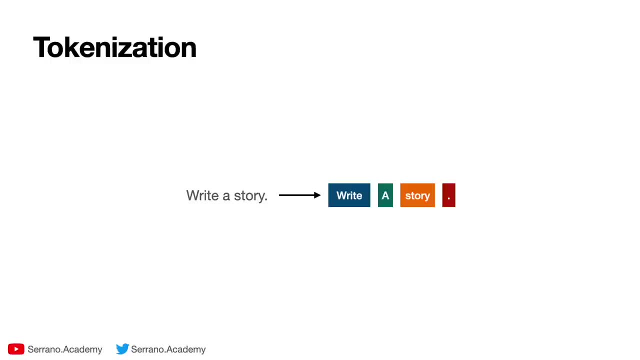 signs also have tokens. sometimes you will also have tokens that are broken into a bunch of words for the beginning and the end of a sentence. however, some words like doesn't get broken into two tokens: the token for does and the token for int. there's a whole science into building good. 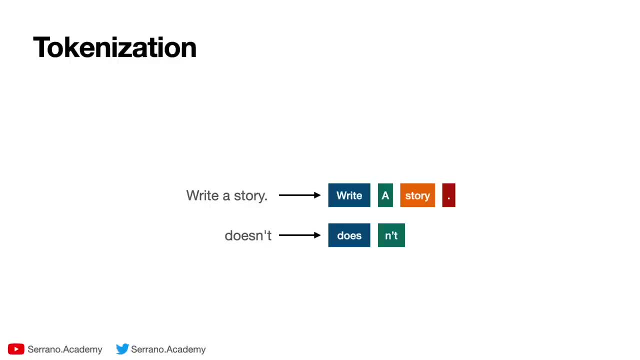 tokens and i'm not going to elaborate here. but if you want to learn all about tokens, i want to recommend you this video from jay alomar, called: did the llm even see what you typed? which is also a chapter on his great book hands on large language models. 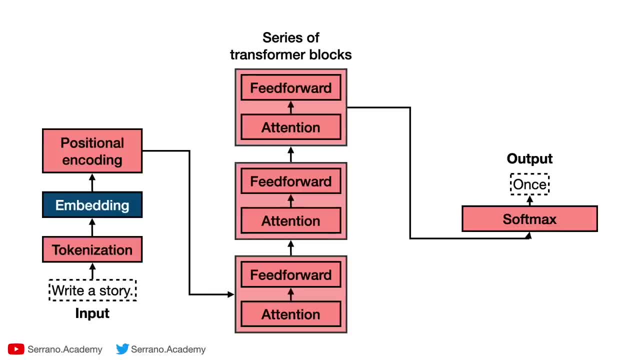 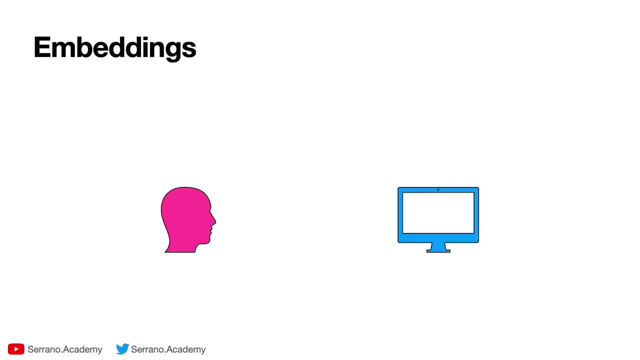 the next step is embedding, and it's right here now. i've talked about embeddings on the previous two videos on attention, but i'll tell you a brief summary here. so embeddings are the most important part of a large language model, because it's really where the translation happens from humans who speak in words. 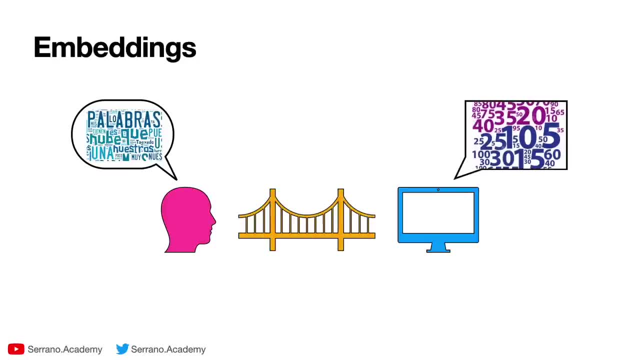 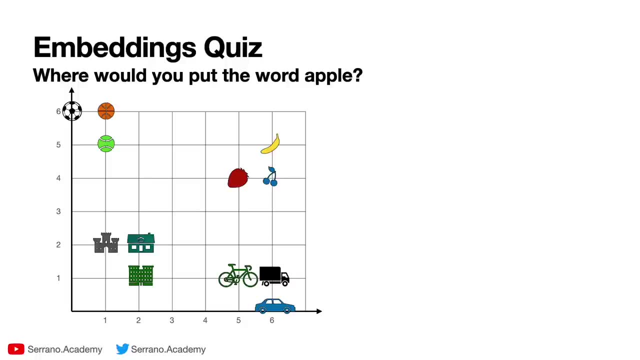 to computers who speak in numbers. the stronger this bridge is, the better large language models are, and the bridge is exactly an embedding. if you recall from the previous video, we had a quiz where the question is: where would you put the word apple? so here we have all the coordinates of the. 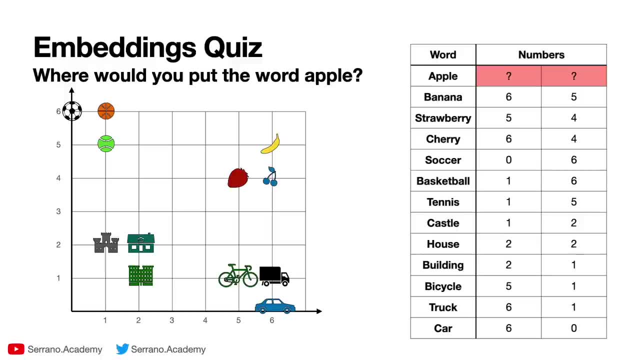 word apple in the first place, where the first number is the horizontal coordinate and the second one the vertical coordinate, and the questions: where would you put apple in position a, b or c? and the answer was c because it should go around the fruits, so a good place for apple would. 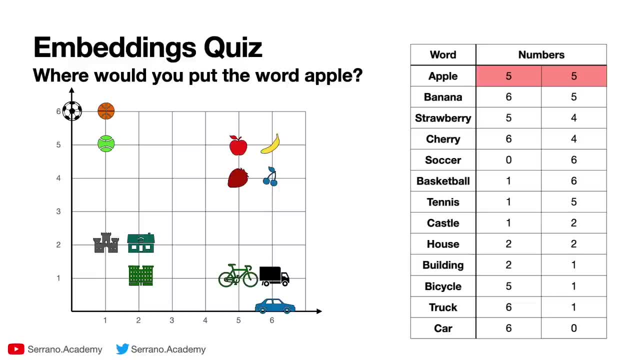 be the coordinates: five, five. now, that's as much as we talked about embeddings, and we also mentioned that you don't just associate them to two numbers, you can associate them to thousands of numbers. but the point is that similar words get sent to similar numbers and in some way the embedding is a bit of a twist. 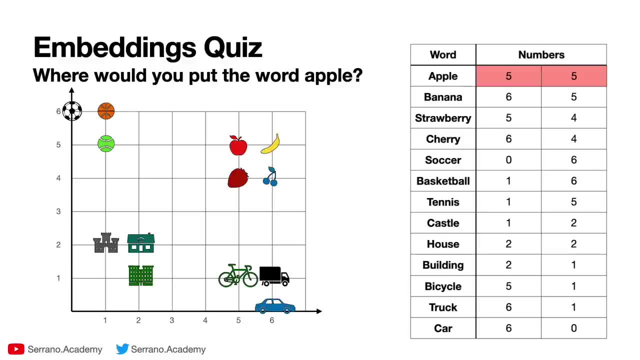 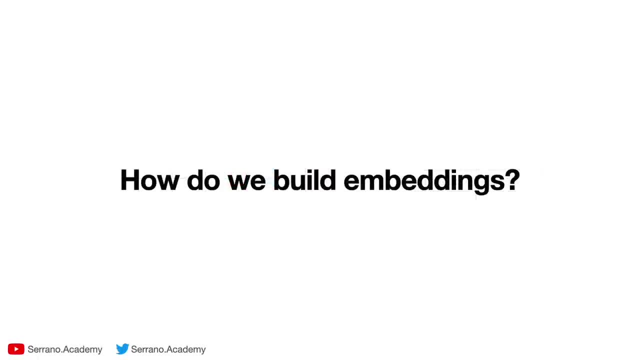 in the description of the word, so every coordinate actually means something, but here we can get a little further. actually, how do you think we build embeddings, and i encourage you to pause this video and think about it. there are many ways, and i'm going to show you one that actually has to do. 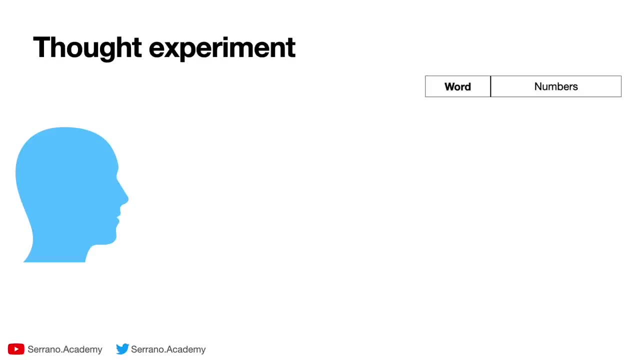 with neural networks. so bear with me. i'd like to think of the following thought experiment. imagine that you actually want to associate numbers to every single word. how do you do it? well, let's say we are going to pick three sensors. Ah, correct, we will project more powers of resistance. 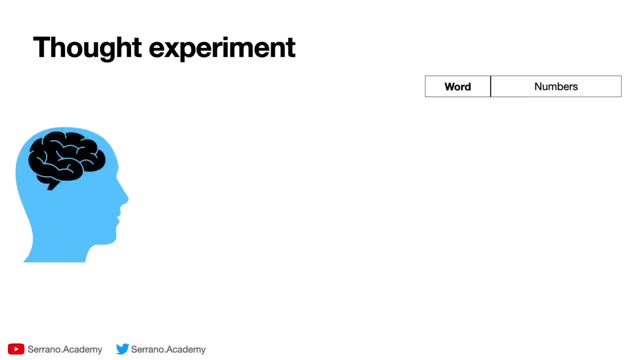 in these regions. Okay, so what we are going to do here is to put these two sensors in the strawberry anymore, literally, that's what I'm going to say. we're going to stop and then put on both sensors to try to use бывает our brain, and these are different challenges, and if we are going to do, 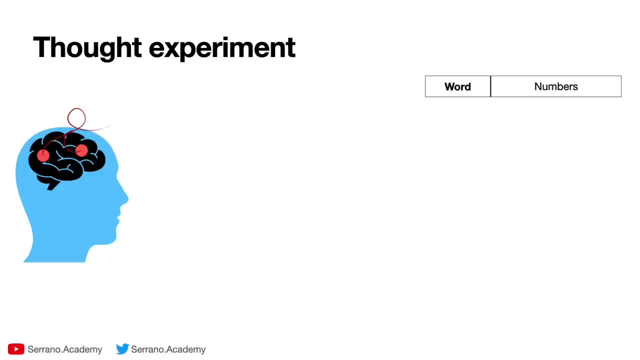 it. anyway, I'm going to take a lot of space and it really looks like a lot, of, a lot of sense but c some activity on that part of the brain In particular. maybe if we can get it to measure the activity on one brain cell, that would be wonderful. But let's just say it measures. 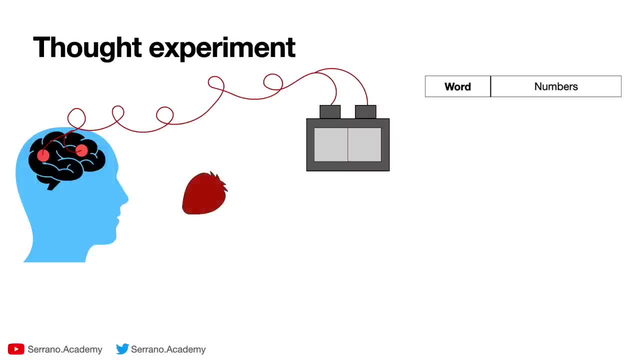 something. Now, in front of the subject we put a strawberry and then we measure what each of the sensors record. Let's say, the first one records a 5, and then the second one records a 4.. That's our embedding. So for the word strawberry, we associate it with the numbers 5 and 4.. 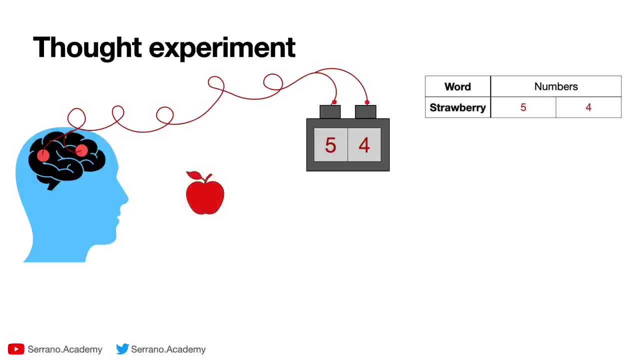 Now what do you think happens if we change the strawberry to an apple and measure the same thing? Some numbers will come out and maybe it's 5, 5.. So we record that the embedding for apple is 5, 5.. Now, if we put a castle instead, then some numbers will come out and let's say they're 2. 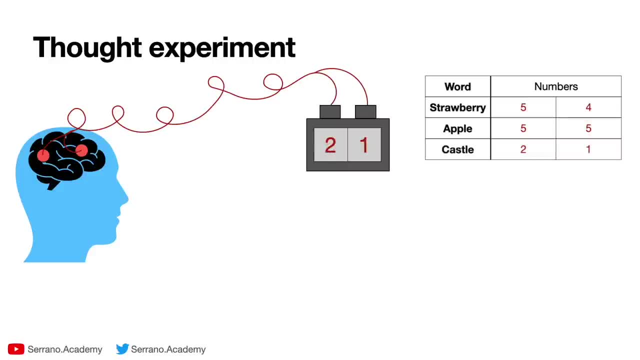 and 1.. So we record 2 and 1 as the embedding for castle. Now, as I said, I don't know any neuroscience, but I imagine that a strawberry and an apple, being similar, must fire similar places in the brain, whereas a castle would fire different places. Therefore, the numbers. 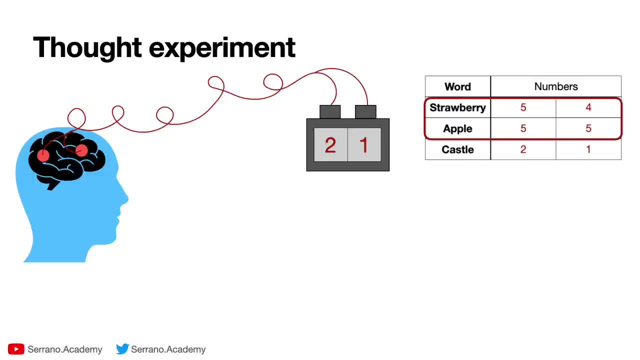 associated to strawberry and apple are likely to be the same. So we record that the embedding for castle is likely to be similar and the numbers associated to castle are likely to be different than these two, So we have pretty much an embedding. I like to imagine that somewhere in 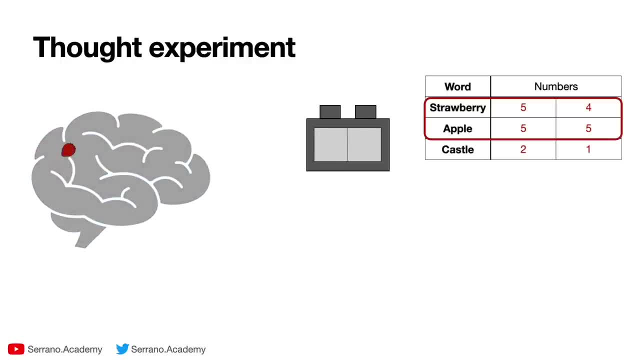 the brain the words are located and somewhere. strawberry and apple are close by and castle is far away, And this is how I imagine an embedding. Now, of course, we don't have subjects with brains to experiment and to build embeddings like that, But what's the closest thing we have to a brain? 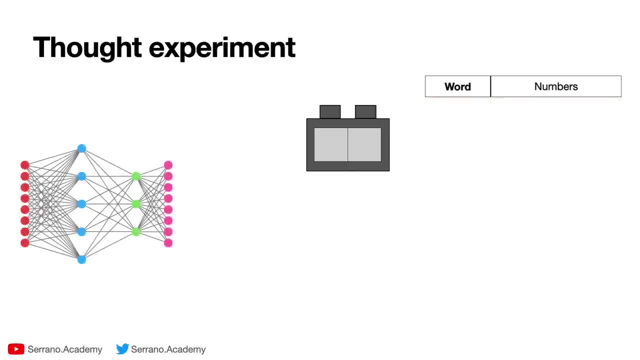 in machine learning. Well, we have a neural network which loosely emulates the brain. So let's try this experiment on a neural network. Let's show it a strawberry. What does it mean to show it a strawberry? Well, this was a neural network that takes a sentence and builds the next. 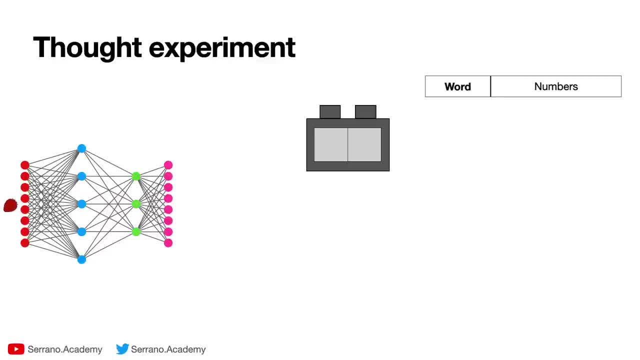 word. So let's just feed the word strawberry to it and see what comes out. Maybe the next word comes out as is or ate or delicious, It doesn't matter. It doesn't really matter what comes out. The pink layer doesn't really matter. Let's take a look at the green layer and put our sensors. 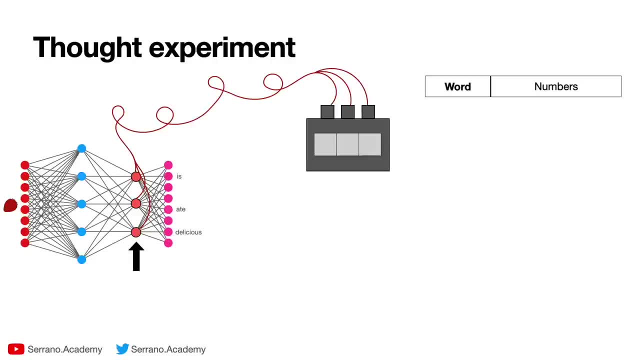 there. So let's make a sentence that says: strawberry and apple are close by and castle is far away. So let's measure what numbers came out of here when making that prediction, And let's say that the numbers- for example, one, three and two- came out. Well, that's going to be the embedding. 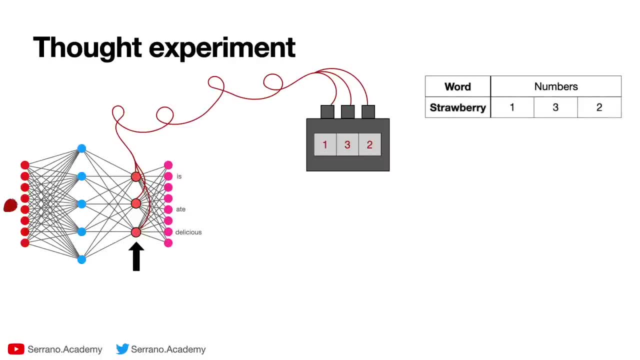 for strawberry, It's going to be one, three and two. Now let's do something similar and put an apple And let's say the numbers 1.1,, 2.9, and 2.2 came out, which are similar to the words for. 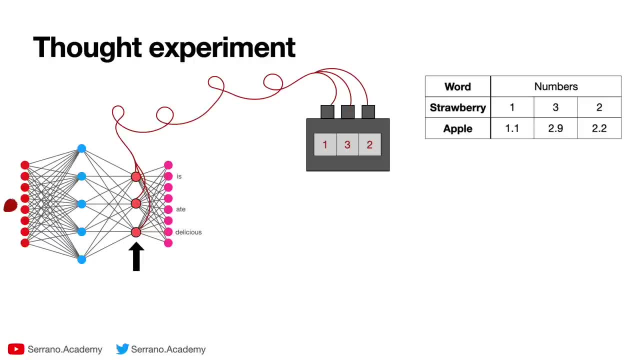 strawberry. Why? Because the reaction that a neural network has to strawberry is similar to the one it has for apple, because the same words, or very similar words, are similar to the one it has for apple. So let's say, the numbers 1.1,, 2.9, and 2.2 came out. Well, that's going to be the embedding. 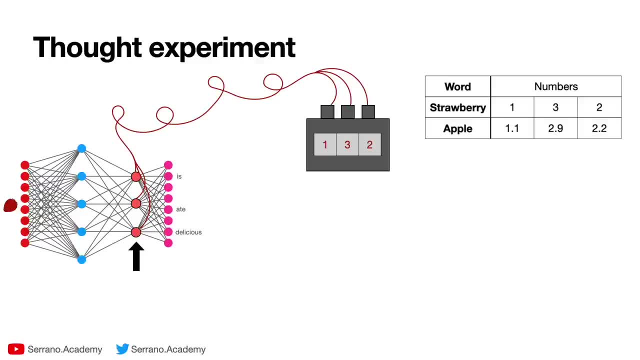 for strawberry. Why? Because the same words would come out. So one would imagine that in the previous layer, whatever numbers came in must be pretty similar. And remember that the neural network has layers and each layer understands deeper and deeper properties of the word. So the 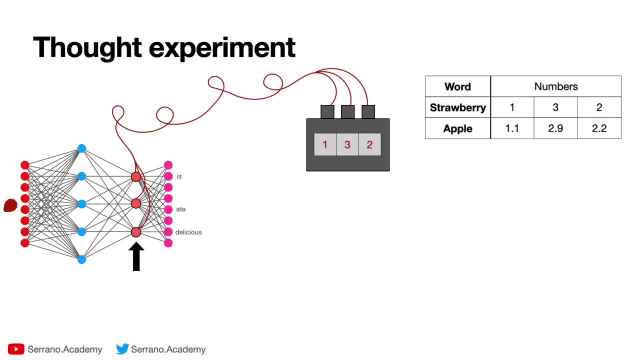 penultimate layer has to understand the word pretty well. Therefore, the three numbers coming out of the penultimate layer in this neural network must be similar for strawberry and apple and must be different for castle. Maybe for castle they are 7, minus 5.4, and 0.4.. In other words, when we 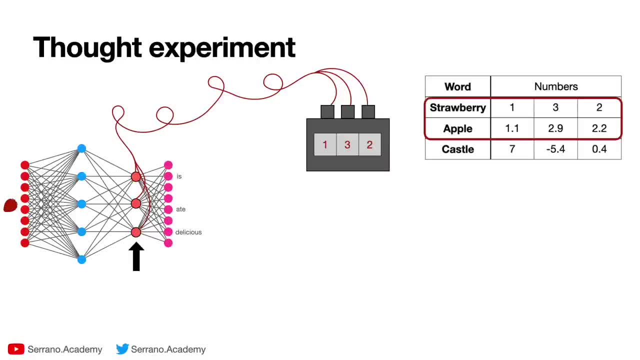 train a neural network to guess the next word, it kind of has to understand words pretty well. And understanding words pretty well means that these layers must capture properties of the word and the penultimate is going to capture some pretty deep properties. And therefore, if we train, 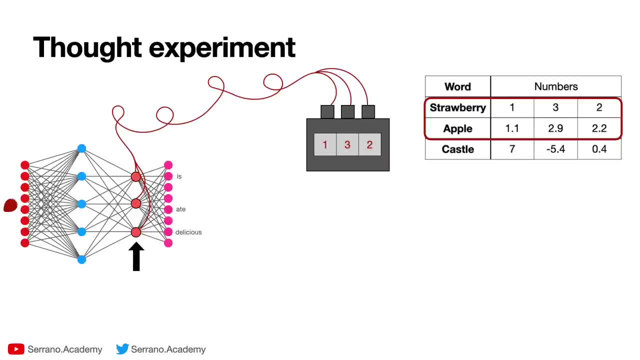 a neural network. well, for free, we get a pretty good embedding by simply looking at the penultimate layer. Now, in this case, the layer has three nodes, but it can have 100 or thousands, And so, therefore, we can create embeddings of thousands of numbers like this. This is a pretty common. 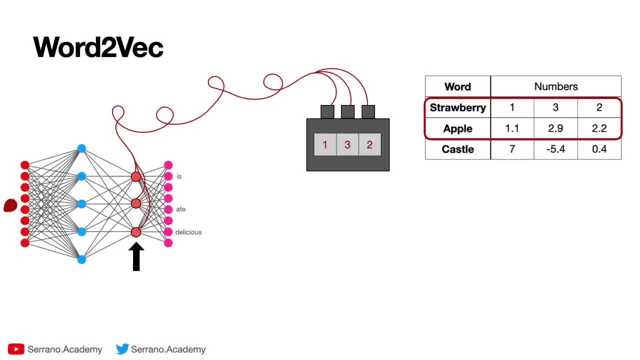 method to find embeddings, and it's called word2vec. Why word2vec? Because it sends the words to vectors. As I said, there are many ways to create embeddings, but those embeddings created with neural networks are some of the most powerful ones. 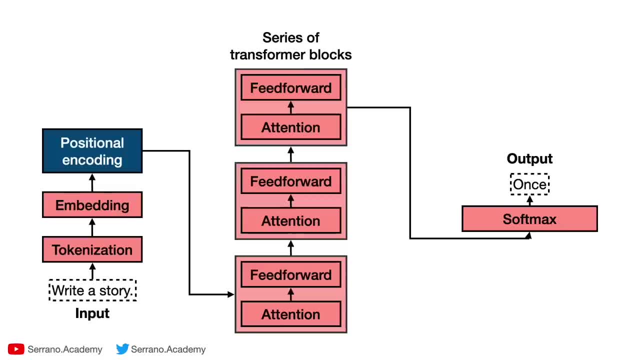 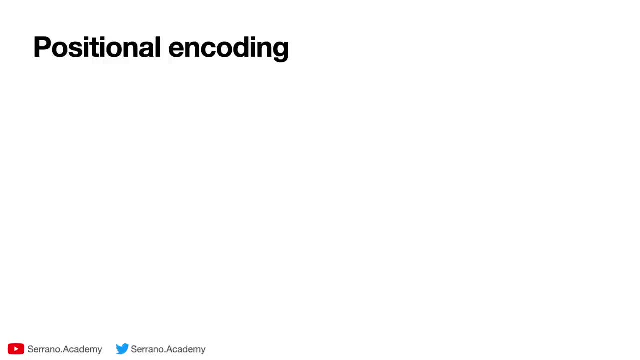 Now the next step is positional encoding. Positional encoding is very important because it takes care of order. Now, to be honest, positional encoding looks a little strange to me because it doesn't really take care of the order in a way that captures the semantics. It just kind of 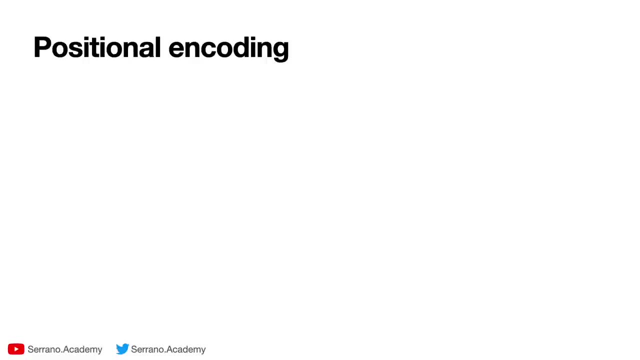 differentiates sentences that have different order, But at the end of the day it works well, so we use it. So let's say you have the sentence write a story period that has four tokens, And that's not the same as saying story period I write. That makes no sense. But now imagine that. 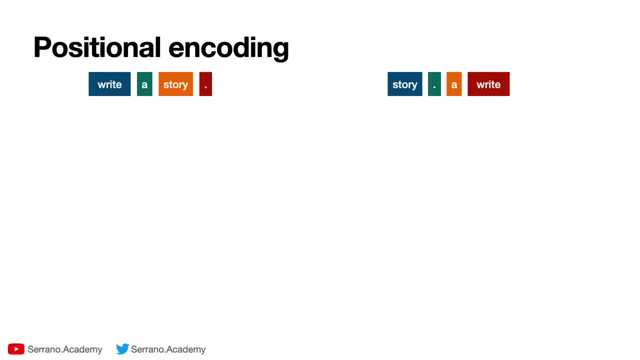 you make it a story period and you have a story period that has four tokens And that's not the same as saying story period. I write That makes no sense. But now imagine that you make it into something that makes sense by reorganizing the words and the answer would be different. So at the end of the 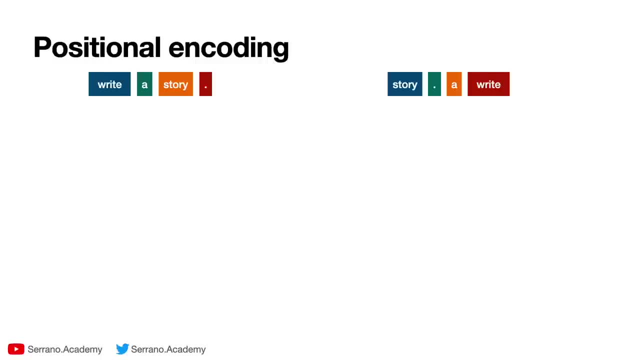 day. the order of the words actually matters, So we would not want to feed the same thing into a neural network with the sentence on the left and with the sentence on the right. So what do we do? Well, we just learned embeddings, So let's look at what the embedding looks for these two sentences. 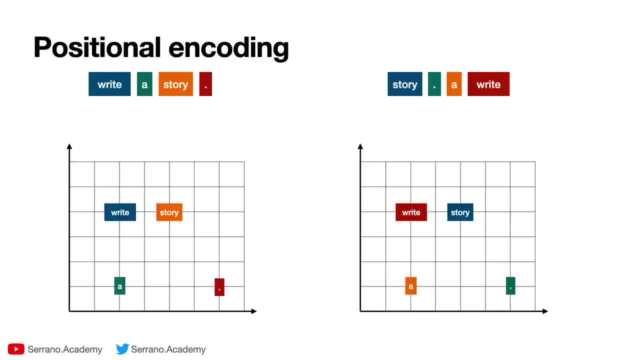 Let's say that this is where the words are located in the embedding, And what we're going to do is perturb each of the words slightly. So let's say that this is where the words are located in the, in such a way that the first word gets perturbed in the same way, then the second word gets perturbed. 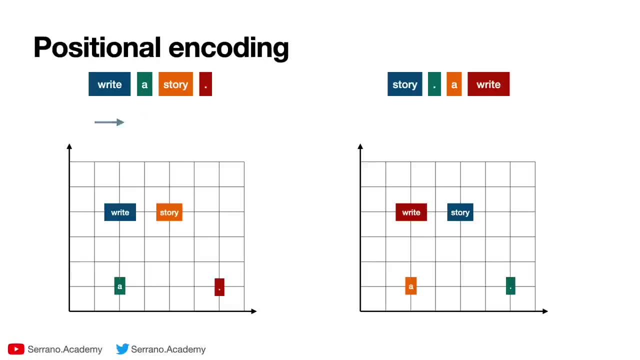 in a different way, etc. etc. So I'm going to symbolize that by arrows: the first word gets moved to the right, the second one up, the third one diagonally to the left and the fourth one a little bit more towards the left. it doesn't really matter. The fact is that we are moving the words. 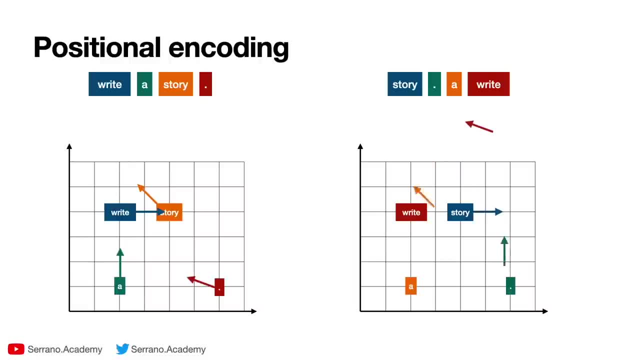 in this direction. And for the second sentence, we're doing the same thing Now, when the words move, now we're going to move the words in the same direction. So let's say that this is where we get different embeddings for these two sentences And, as I said, there's no semantics. 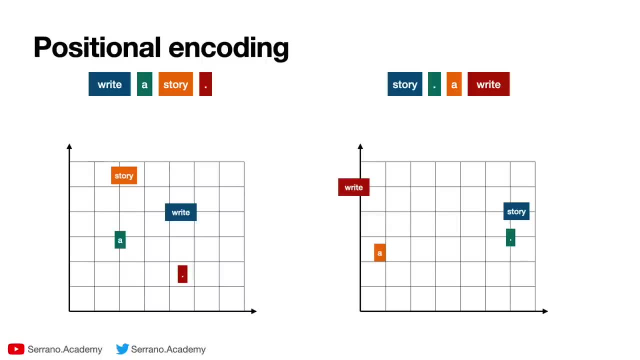 here it's really adding different numbers to the first word, the second word, the third word, the fourth word, etc. in such a way that now the embedding captures order in some way And then the neural network would take care of learning this order more. I understand if it's not as satisfying. 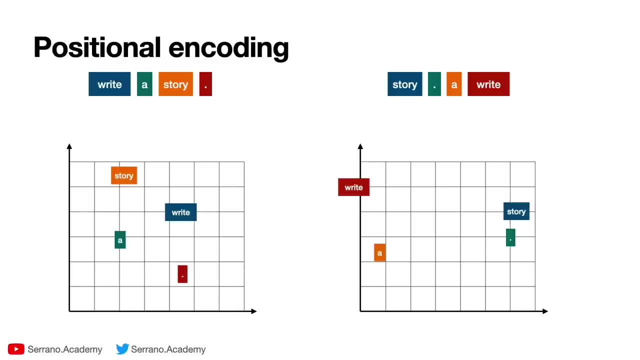 as you wanted it to be, But it works really well. And now these arrows. what is the rule for these arrows? Well, the reason I'm not being more specific is because they change a lot. I've seen them using sines and cosines, I've seen them using exponential function, but better and better. 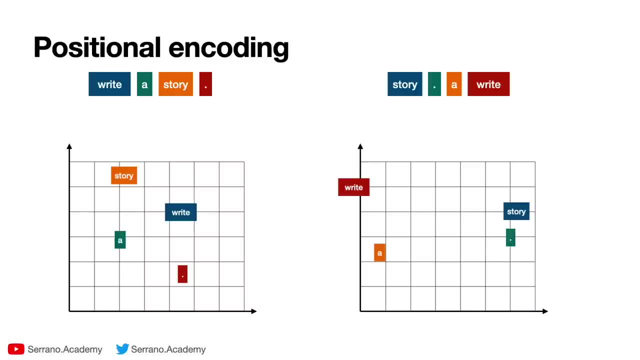 positional encoding functions keep coming out, So maybe by the time you see this video, there's a completely different one. All you need to know is that these numbers normally follow a sequence. So, for example, this sequence of arrows that rotate slower and slower every time are one that 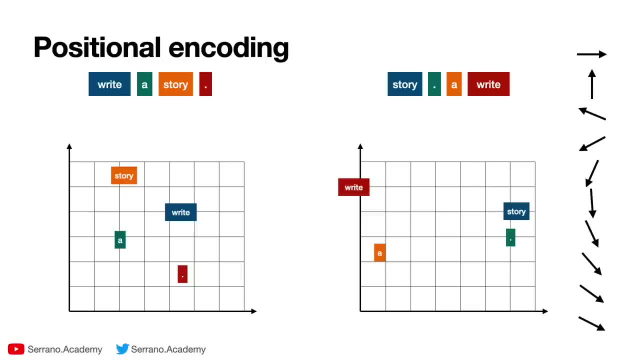 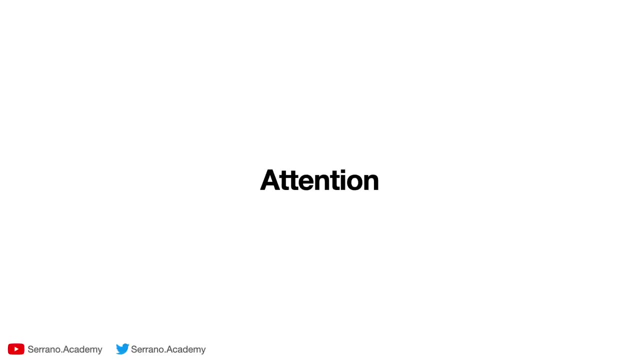 works as positional encoding, But if you want to remember one thing about position encoding, you some kind of sequence that you add to each one of the words in the sentence in order to move them around and perturb the order. Now the next step is attention, which is crucial in the transformer. 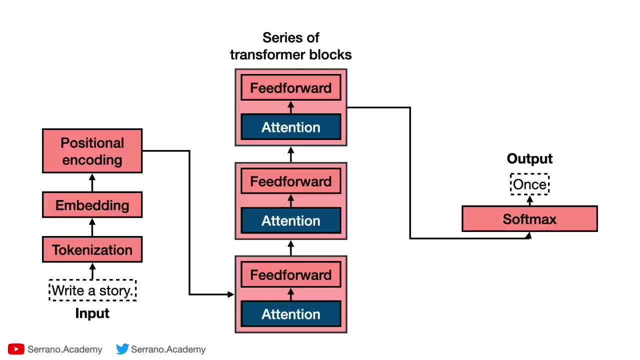 models. As a matter of fact, it's really the step that made them work really well, because it's the step that really captures the context. Attention can appear many times in the architecture, because it appears in each one of the transformer blocks, followed by some feed forward layers, and I know 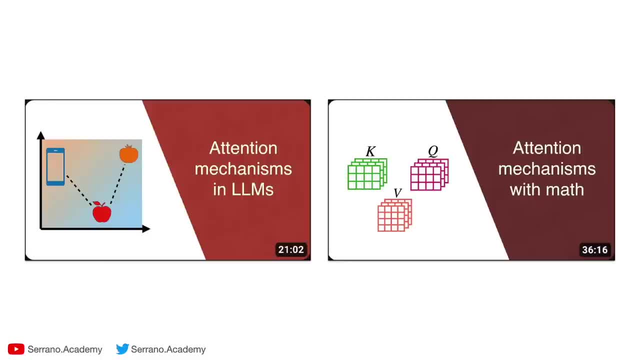 that I already talked about attention for two long videos which I really recommend you to watch if you haven't, but I can't help it. I love talking about attention, and so I'm going to tell you a little bit more about it here. So, to summarize, if you have an embedding, let's say you have all the 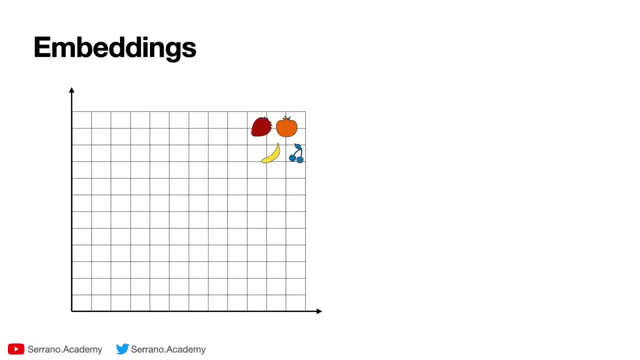 fruits around here you have a strawberry, an orange banana and cherry, and here you have a bunch of computer brands and computer words. you have laptops, smartphone, android and microsoft. The question is, where would you put the word apple? Well, it kind of belongs to both, so it's. 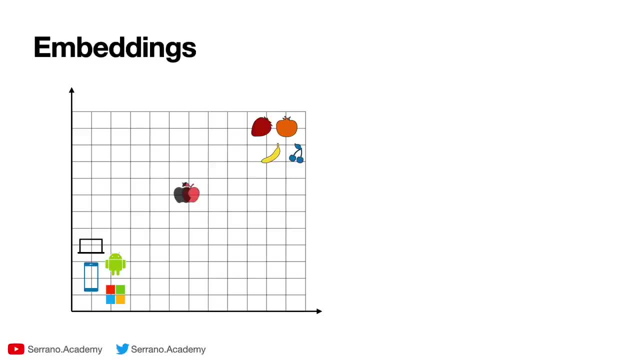 hard to tell, so the best you can do is to put it somewhere in the middle, and that says that, no matter how good embedding is, there are some things it cannot capture because it's not going to know where to put apple. So we are forced to use the context, and in the context we have to look at the 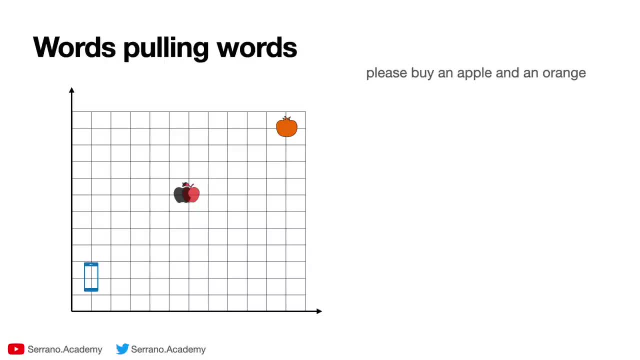 sentence. if you have the sentence please buy an apple and an orange, then apple means a fruit. and if you have the sentence apple and violet a new phone, then you're talking about the technology brand. So that means the word apple gets influenced by the word apple and violet. So if you have the 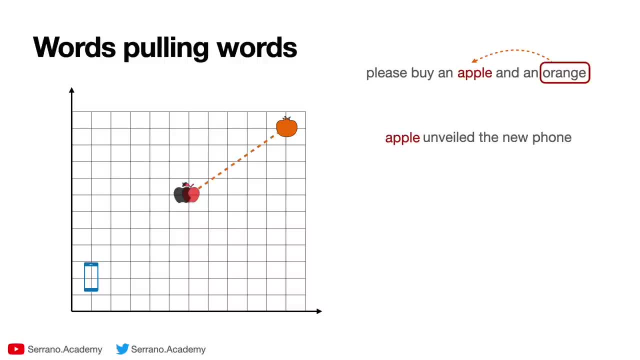 word orange in the first sentence, which means that the orange has a gravitational pull over the word apple and pulls it closer to it, and for the second sentence, the word phone affects the word apple, so the phone pulls the word apple here, and therefore now we're not going to use the coordinates of the. 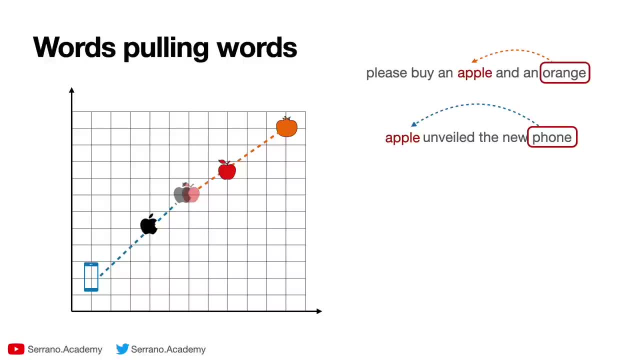 apple in the middle. we're going to use for the first sentence the coordinates of the apple on the top right that is pulled by the orange, and in the second sentence we're going to use the coordinates for apple when it's pulled pulled by the word phone. so I like to imagine attention as a gravitational pull between words. 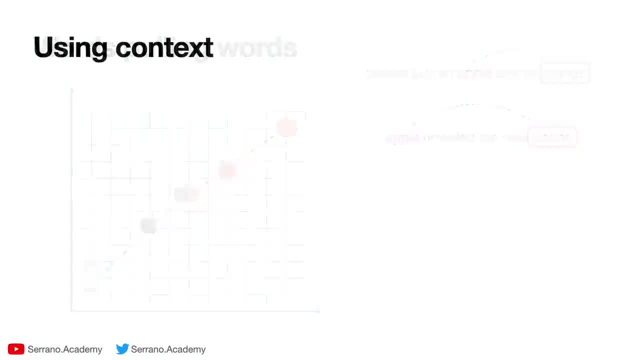 that appear in the same sentence or in the same context. Now, speaking about context, there is this example that I really like. Imagine the sentence: the bear ate the honey. because it was blank, we haven't finished the sentence. The question for you is: what does the word it describe? Is it talking? 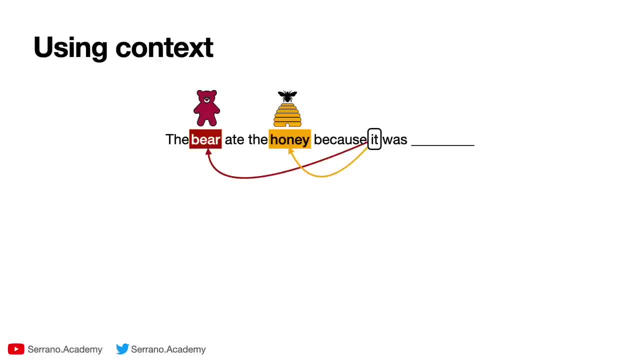 about the bear or is it talking about honey? Well, we don't know, because it depends on the next word. it could really be either one. In particular, if the blank word is hungry, the bear ate the honey because it was hungry, then we're definitely talking about the bear. but if the sentence says the bear ate the honey because it- 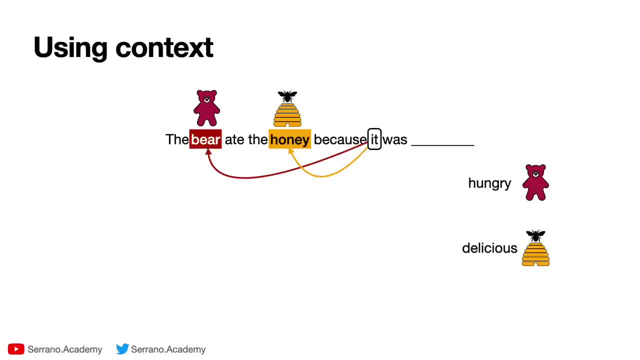 was delicious, then we're definitely talking about the honey. So that last word is the one that makes a difference. Now, how do we explain this? using attention and gravitational pull between words? Well, let's look at all the words and let's put them in an embedding, like we know how to do, and 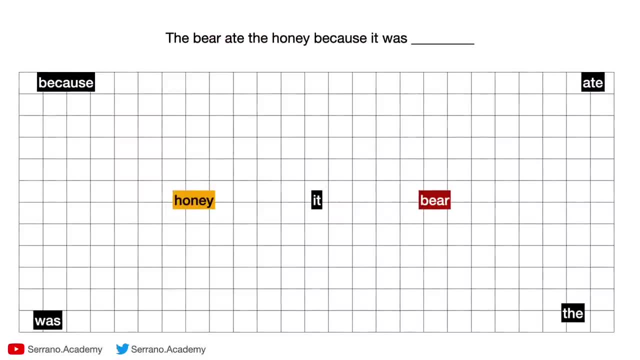 let's forget about the last word. So let's see what happens. before we've got the last word, We've reached the end of the sentence. In this embedding, words are similar if they appear in the same context many times, So two words that are likely to be replaceable are similar. So for 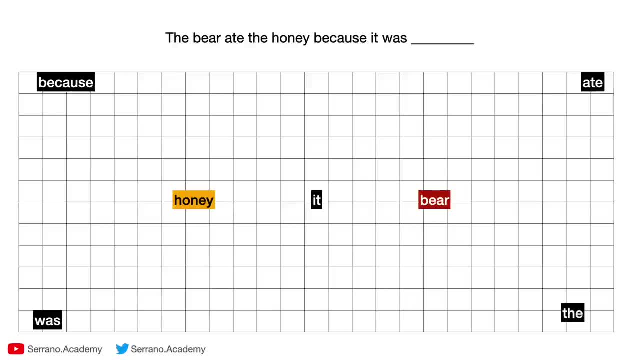 example, it and bear are similar because many times a sentence could have the word it and could also have the word bear, and the same thing happens with it and honey. They are similar because I could have sentences with the word it and the same sentence with the word honey. Therefore, these: 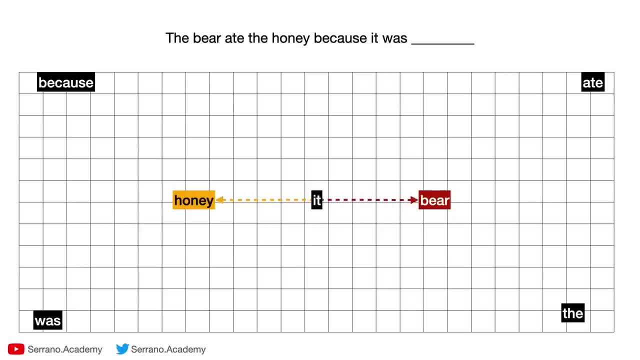 two words exert strong gravitational pull to the word it. All the other words also exert gravitational pull, but not as strong because they're not as similar. So let's forget about them and let's only think of the word it being pulled towards bear and towards honey, but at equal. 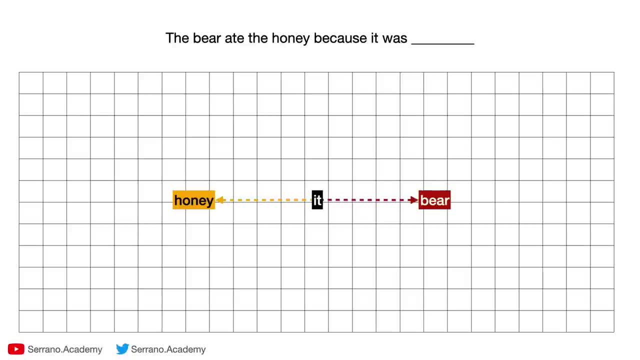 amounts because it's kind of similar to both. So it kind of stays in between, gets here in a game of tug of war, but it's between the two And if we don't know the end of the sentence then it can't really gravitate towards bear or towards honey. However, once we know the next word, something 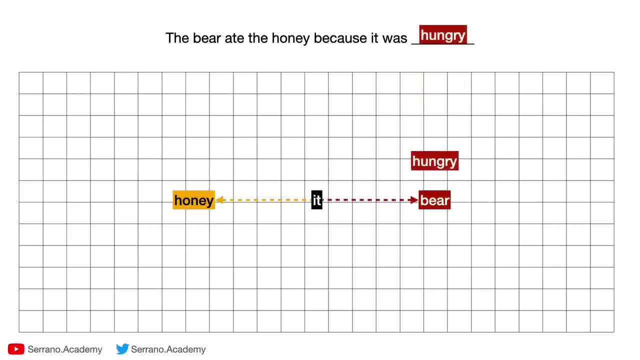 next word is hungry. Well, hungry is similar to bear more than hungry, similar to honey, because hungry will be often describing a bear. Therefore, now we have two words pulling in the bear direction and one pulling in the honey direction, and therefore it will gravitate towards bear and 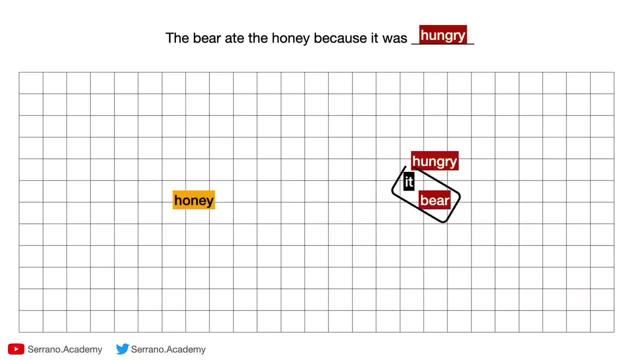 hungry in particular, be closer to bear. So we know that it describes the word bear. On the other hand, if the word at the end of the sentence is delicious, well, delicious is much closer to honey than to bear, because delicious describes the honey And delicious is going to pull the word it. So now we have two words pulling towards honey and 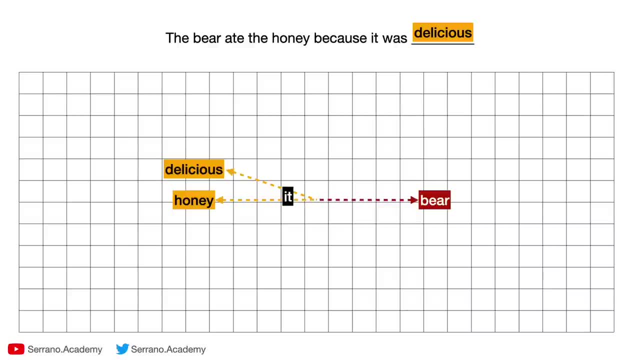 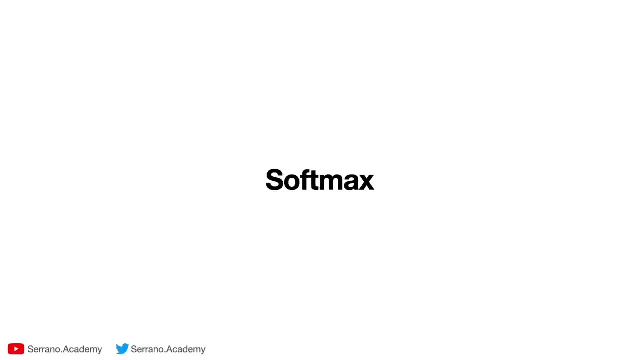 one towards bear. So it goes in this direction And after many iterations it's going to go very close to the word honey and therefore we know that it describes the word honey. And this is how attention works. Now I'm going to skip ahead a little bit and tell you about the softmax. Now 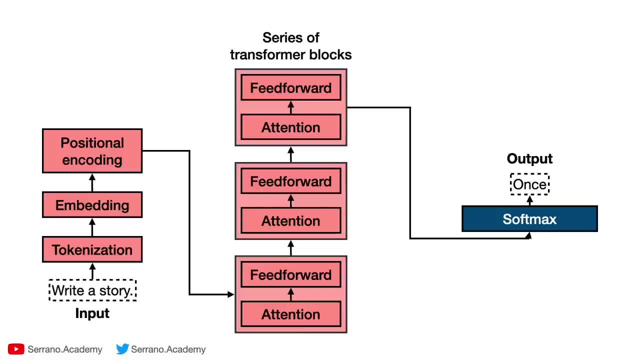 I haven't told the whole story about the series of transformer blocks, but assume that it's a big, huge neural network. So let's start with the softmax. So let's start with the softmax. So we have this kind of a new neural network that predicts the next word. Now, we saw that before. 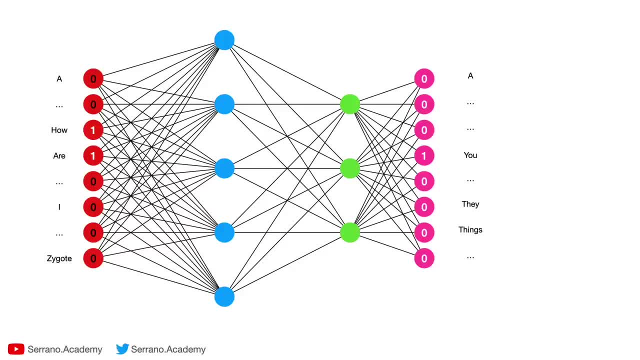 right, because we have this big neural network that is used to predict the next word or sentence. If I input, how are it will output you. Now, we don't exactly want that. we don't want a deterministic answer. We don't want that every time I say how are it, responds you Because in reality you. 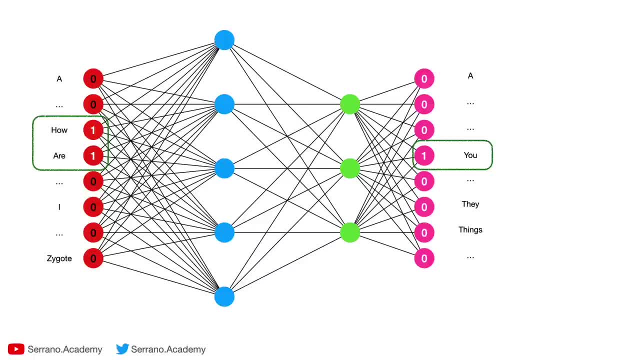 wouldn't want the exact same answer every time you ask a question. you want something probabilistic, something stochastic. So we're just going to add a mini step that makes this interesting to a probability. So, instead of outputting a bunch of zeros and one one for the next word, we're just 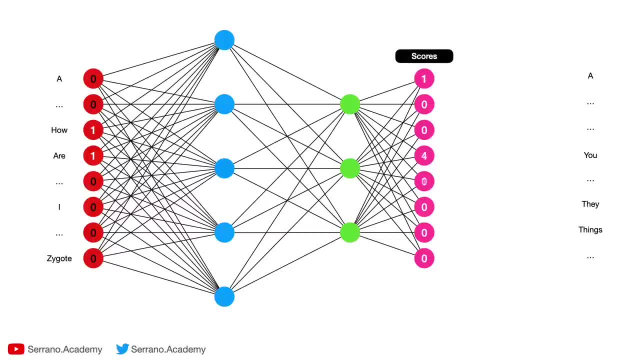 going to make it output some scores, and these scores can be anything. They are high numbers for words that are likely to appear and low numbers, even negative numbers, for words that are very unlikely to appear. Now we would like to turn this into probabilities because at the end, 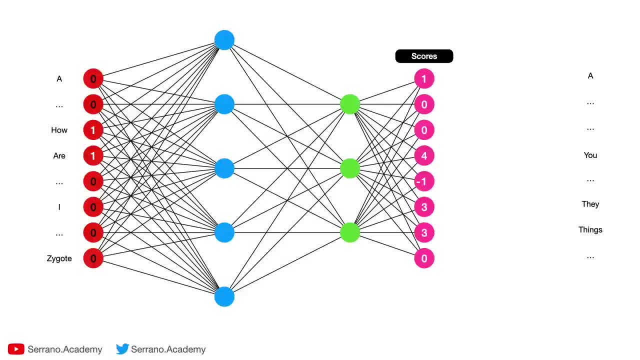 of the day. we would like to draw a word out of a bag, given probabilities, where the words of high scores have higher probabilities and the words with low scores have lower probabilities, because we still want it to be accurate. we just want it to be a little different every time. But what? 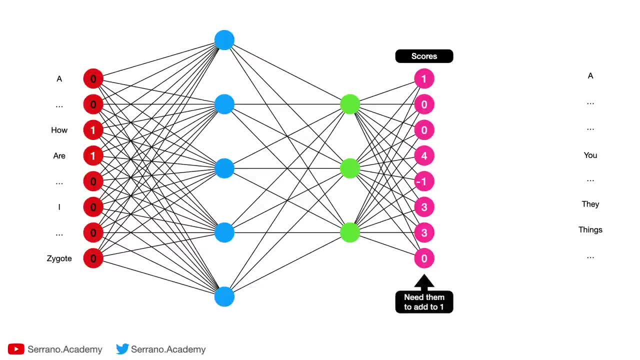 property the probabilities have. Well, all these numbers must add to one. So how do we make all these numbers add to one? Well, one way is to divide them all by the sum. So the sum of these numbers is 10 and therefore, if we divide everything by 10, we get 1 over 10, 0 over 10, etc. etc. etc. and those 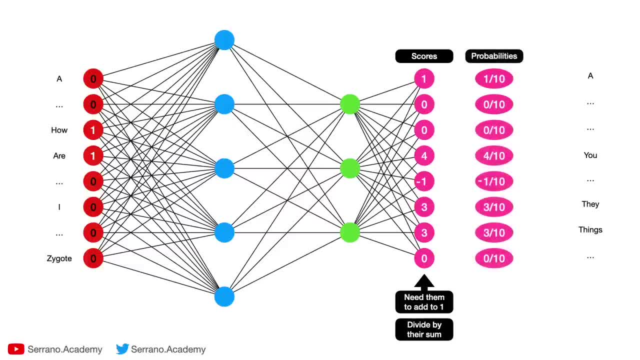 are the probabilities for each word, and then we just draw a word based on these probabilities. So the fourth word, for example, has probability 4 out of 10 and therefore is more likely to appear than, for example, the third word, which has probability 0 out of 10.. 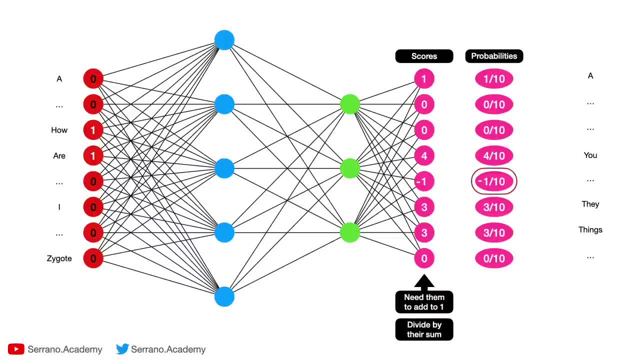 The problem is that we have some negatives and we can't have negative probabilities. Minus 1 over 10 is not a probability, So we actually need these numbers to be positive. What do we do for these numbers to be positive? Well, one very popular way is to raise e to the score, because e to the 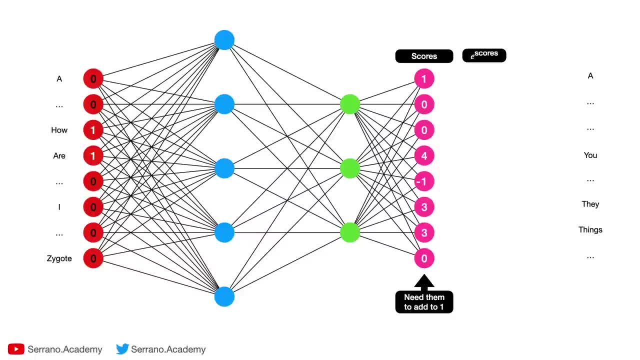 anything is a positive number. We can actually raise 2 or 3 or any number we want, but e works pretty well and this is actually called the softmax function, if you've heard about it. So we take: 1 becomes e to the 1,, 0 becomes e to the 0,. 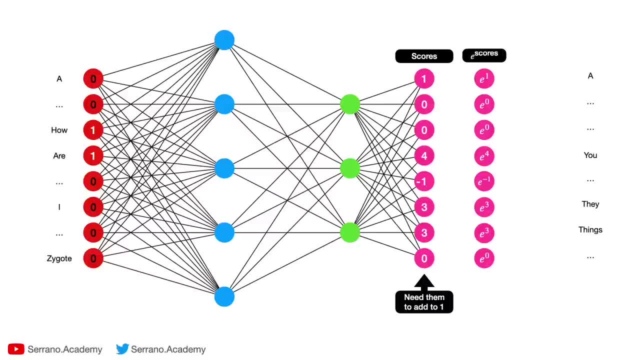 4 becomes e to the 4, minus 1 becomes e to the minus 1, which is okay because e to the minus 1 is a small number, but it's positive. and now we have a bunch of positive numbers and we divide by the sum and when we divide by the sum we get the following probabilities and notice that the 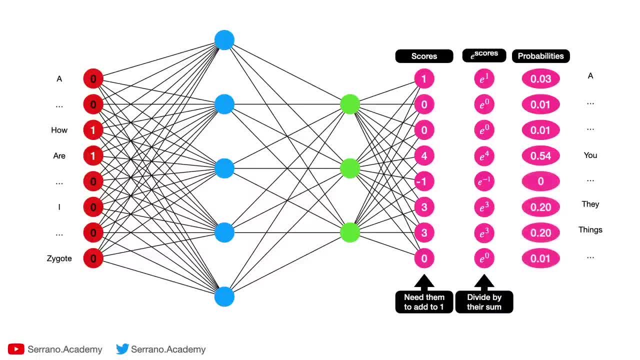 highest one is the one corresponding to 4, which is 0.54.. The lowest one is corresponding to minus 1, which is not 0, but it's so close to 0 that I rounded it to 0. and the higher the score, the higher the probability, and the lower the score, the lower. 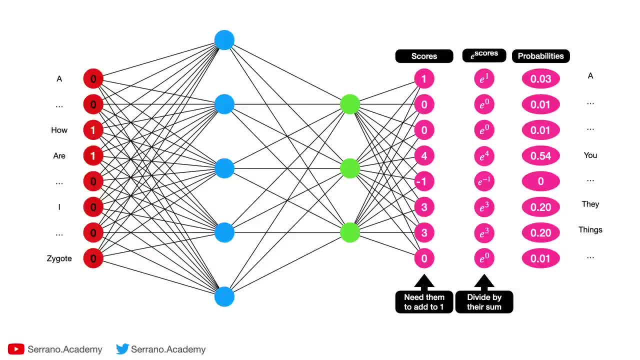 the probability. So we are being faithful to our scores and if we draw a word out of here with these probabilities, well, most likely we're going to get the word you, but we can also get the word they or the word things sometimes. So this is a way to select words out of a probability. 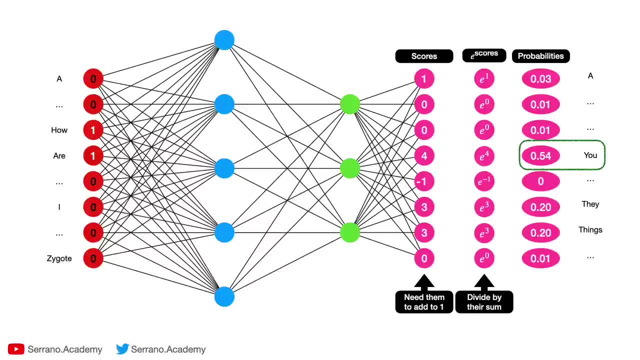 distribution formed by the neural network, in a way that you're always going to get good words coming out according to the input sentence, but you're not always going to get the same ones. Okay, so now that I told you softmax, let's go back a little bit and take a look at the whole. 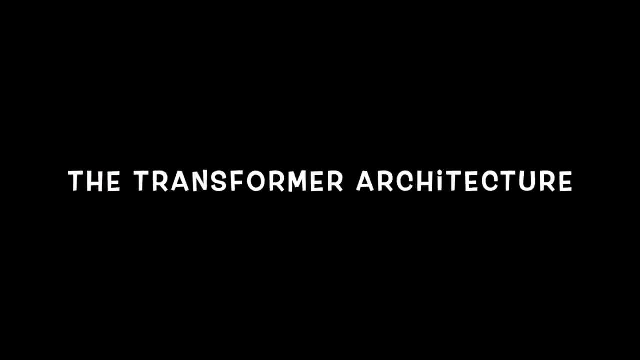 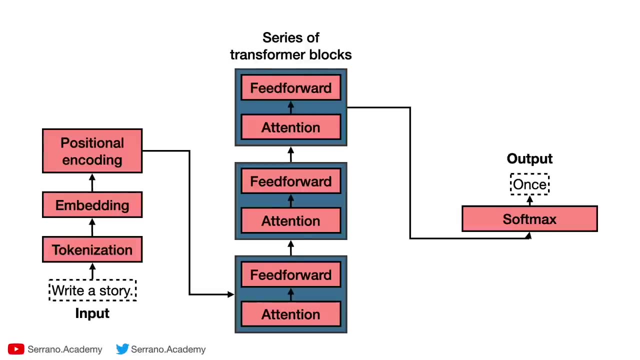 architecture. Okay, so now we have all the parts to build transformer, and the architecture is this. There is one part that is still not super clear, which is a series of transformer blocks formed by attention and feed forward, So this can be multiple ones. there can be. 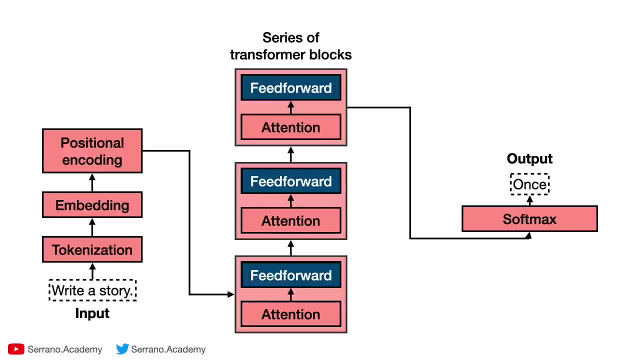 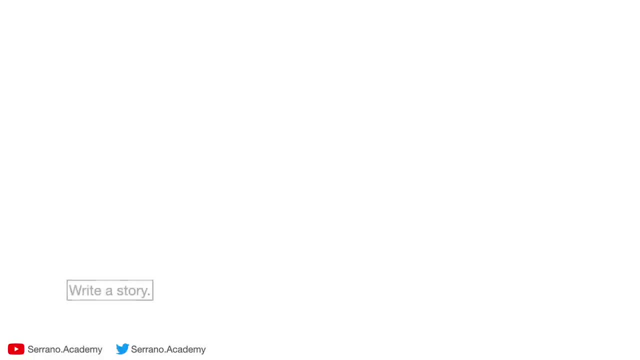 12, it could be more, and at the end of the day, each block has the similar architecture. So to see this clearly, let's go through the whole architecture. First. we start with the input text, which is, let's say, write a story. It goes through tokenization, which means everything becomes a. 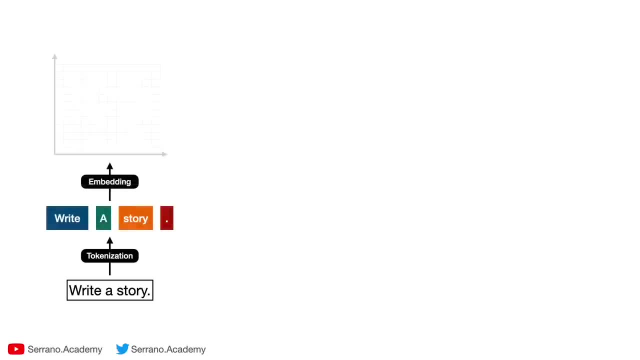 bunch of tokens. Now it goes through an embedding, which means these get put into some big, big space with lots of coordinates. Then we go through positional encoding, which means each one of these words gets disturbed in some different way, In a way that now position gets recorded and two sentences with the same words but in different. 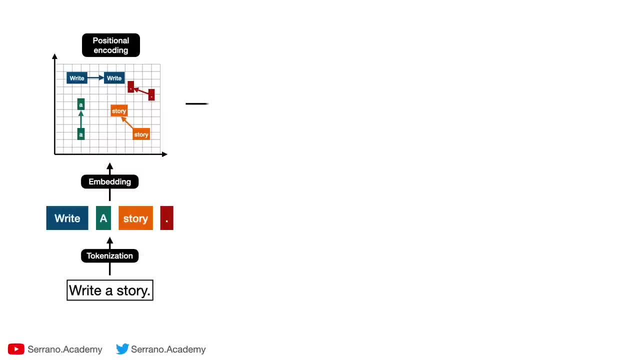 order gets sent to different embeddings. Next, these numbers, these coordinates, are fed to a neural network and that neural network is trained to find the next word in that sentence. However, that neural network is not very good because it still doesn't capture context. This neural network. 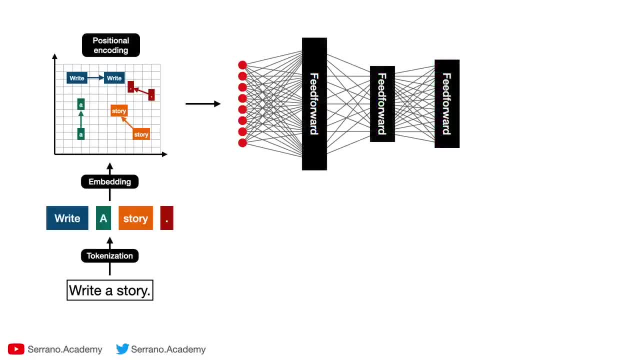 is made by a bunch of feed forward layers. Now what we're going to do is we're going to throw in an attention layer in between each one of these. Now, the feed forward doesn't need to be one layer. it can be multiple layers at a time, but at the end, 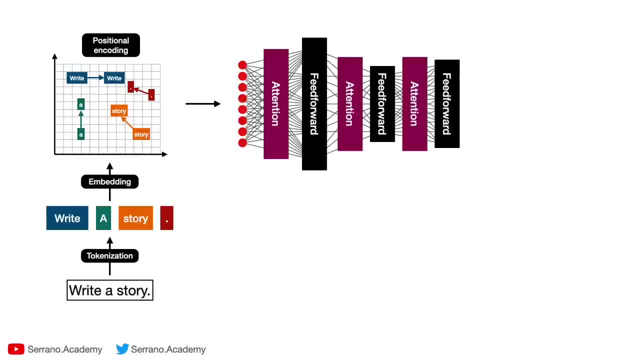 of the day, what we have is that in between each of the feed forward layers, we do one attention step, one gravity step, And if you see the second video on attention, there's actually something called multi-head attention. That's what happens between two feed forward blocks. This part may be sounding. 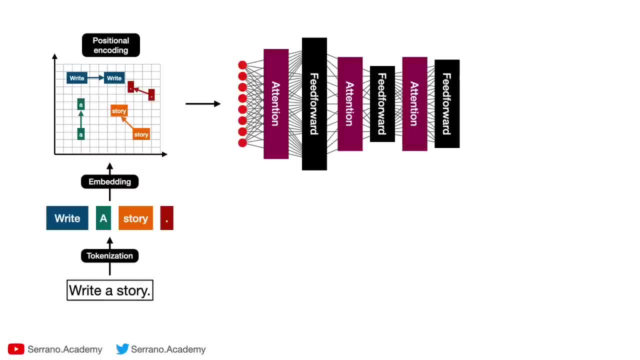 a little abstract, but just imagine a big neural network with a bunch of attention layers thrown in between. So as you train the neural network to guess the next word in between each one of the feed forward layers, you always remember to add context often, And this is going to not give us the 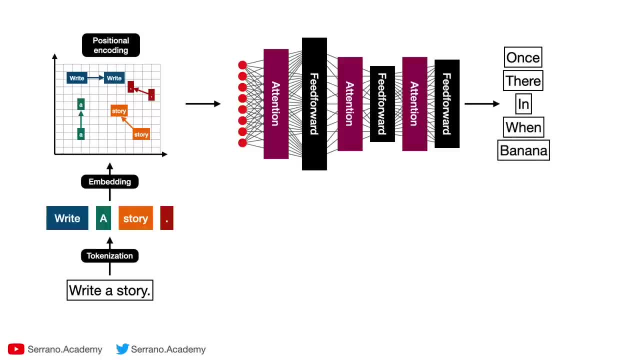 next word, but it's going to give us for every single word in the language it's going to give us, actually for every single token. it's going to give us a score and the softmax is going to give us a probability for each word or for each token. For example, a token could be end of sentence. 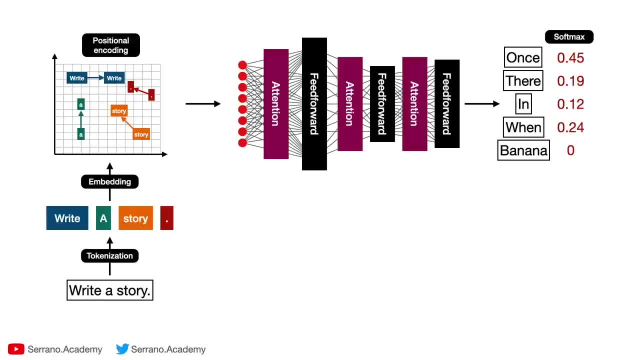 that could be the one that dictates when the transformer basically needs to stop talking. So, from here, the highest probability word is the most likely one to appear, and let's just say that when we draw out of here, then the word once comes out, and so that's the output of the transformer. So all this, 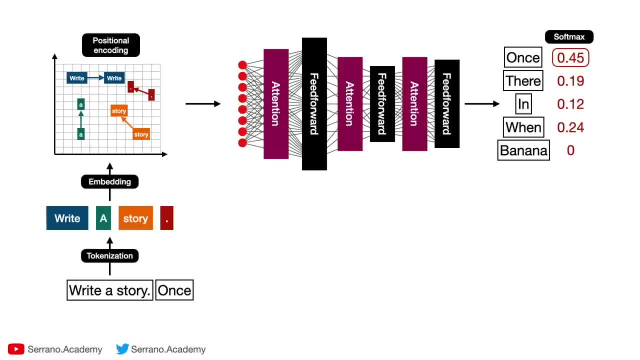 process to guess the next word, But because we've trained it that way, then this word is pretty good because, first of all, position is taken into account, second of all, context is taken into account and the neural network that guesses the next word is pretty strong, because we're talking. 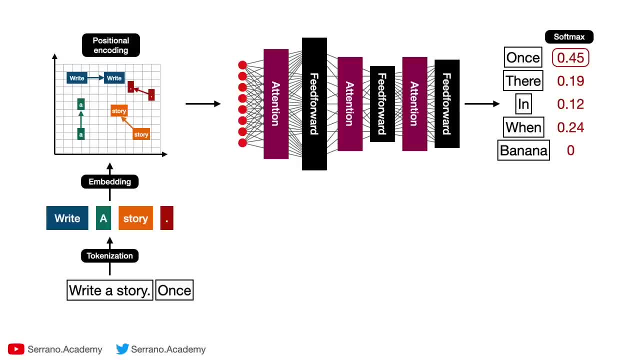 about a huge architecture with lots of nodes, lots of data, So we're going to guess the next word, and that's really what makes transformers so good. So, as you can see, the architecture is not really that complicated. it's really just a big neural network with a bunch of padding and a bunch of boosters. 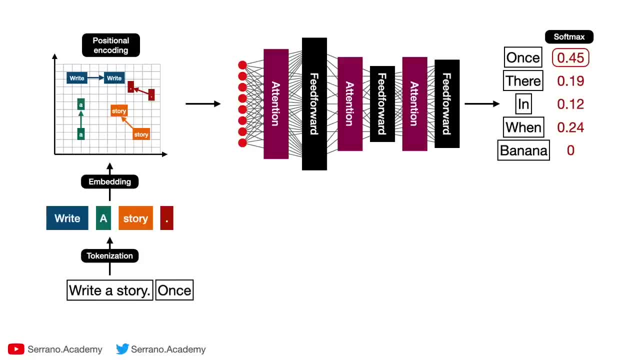 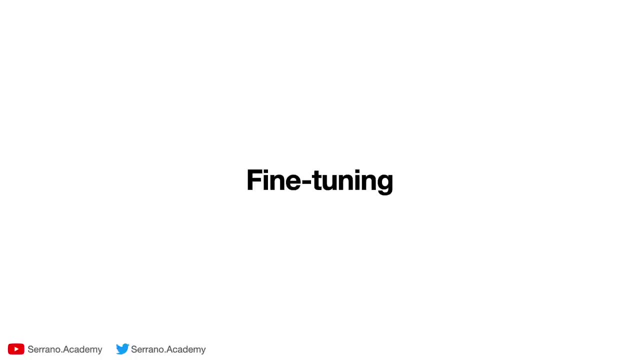 around that make it work really well. And that's it. that's the transformer architecture. And so are we done? yet Well, let me show you some problems that transformer have and also some solutions that I provide. So, as I mentioned before, transform models don't always work as intended. if you sync a 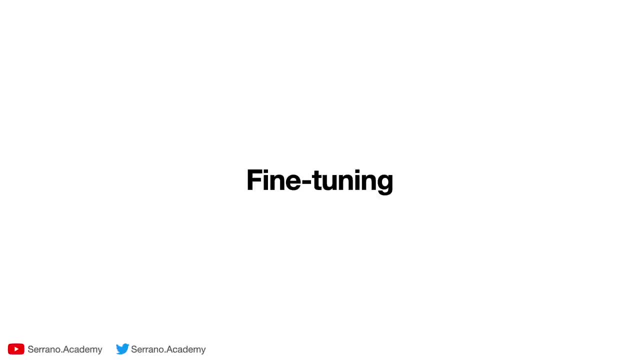 bunch of data sets with a bunch of data sets. So what I'm going to do is I'm going to train them to talk using the entire internet as a data set, And to fix that we have a process called fine tuning. So why wouldn't a model work if it's trained on the internet as a huge data set? Well, maybe because 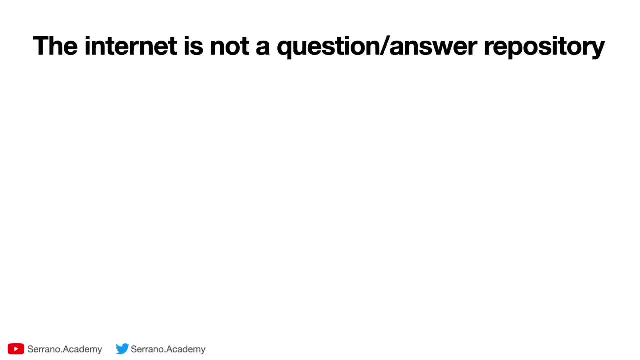 the internet is not exactly the best place for many things. As a matter of fact, the internet is not a question answer repository. For example, if I train the model to guess the next word and I ask it a question: what is the capital of Nigeria? Well, the answer is Abuja. 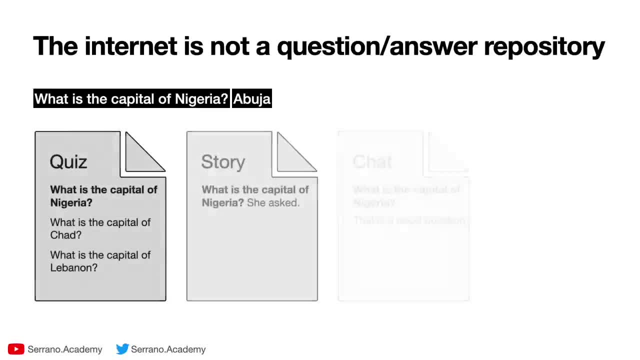 That's a common word. right after that sentence, I could have the internet looking like this And there could be some quizzes where, after what is the capital of Nigeria, the next thing is a question- what is the capital of Chad or what is the capital of Lebanon? And the next word is what? 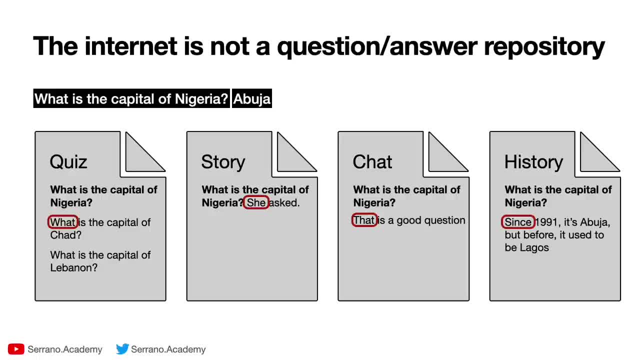 I could also have stories where we have the sentence what is the capital of Nigeria, She asked. In this case, the next word is she. Or it could be a chat where you have the sentence what is the capital of Nigeria and somebody answering that's a good question, in which case the word is that: 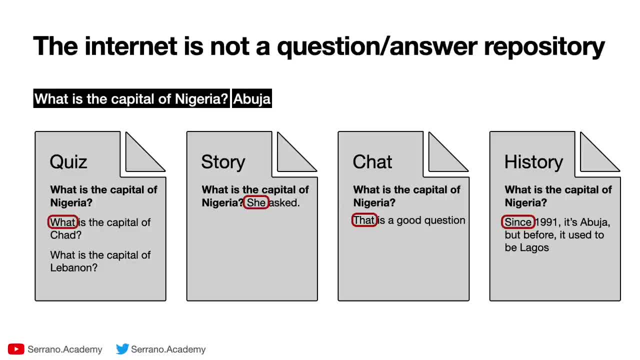 Or I could have a more elaborate answer that doesn't start with the answer. it simply says since 1991, blah, blah, blah, and in that case the word is since. So for the model it's not very clear what the next word should be. and remember that the transform model is not trying to answer questions, it's trying. 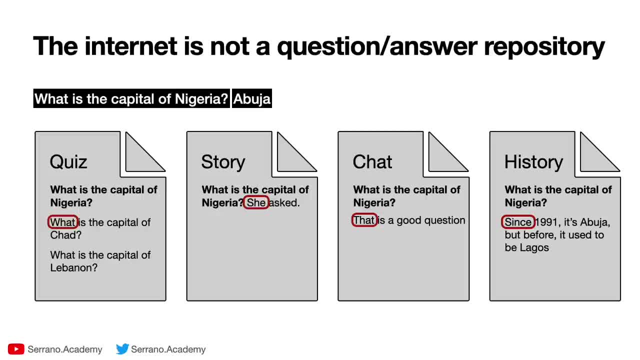 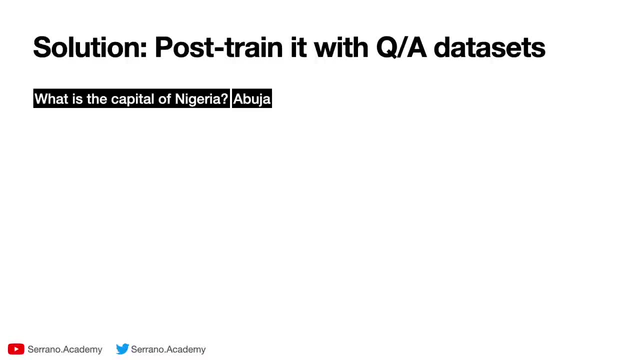 to find the next word. So how do we get the model to know that it's not just the next word that we want, it's the answer. Well, what we have to do is train it on question answer data, So we can use experts to curate a bunch of data. 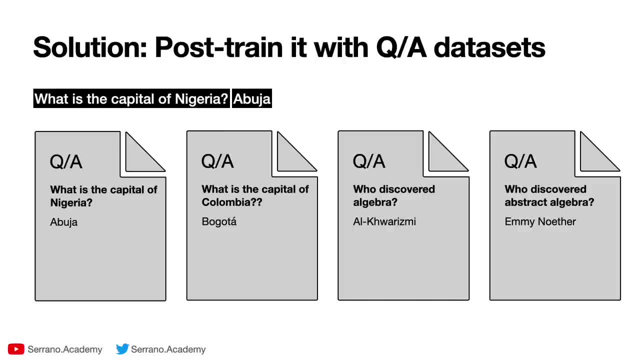 sets that have particular questions and answers, so that the model starts learning that when it gets a question it has to answer with the answer. That's called fine tuning a model and it's a very, very expensive part of training because you actually require people to create custom data sets and you need to be very careful and curate. 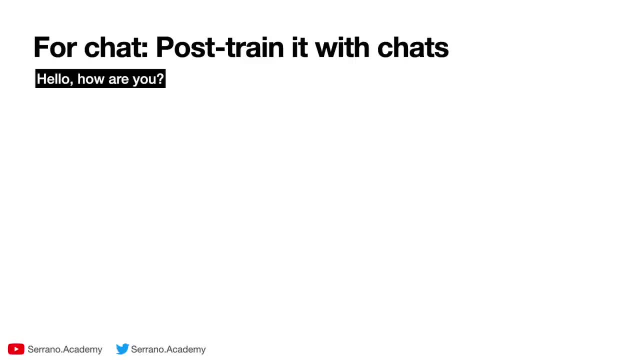 these data sets very well. Now, this is not only for question and answer. if you want the model to actually chat, If you say hello, how are you? and it says good, and you, and then you continue talking and the model continues talking to you, then you need 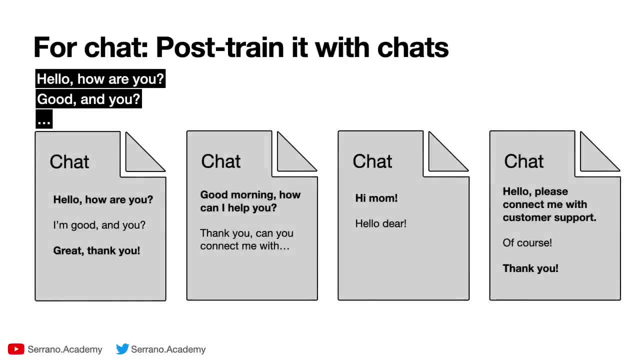 to fine tune the model by post training it with tons and tons and tons of chats. In that way, the model starts learning that if you're talking to it, it has to reply as a person who's chatting back at you, and if you continue talking to it, it should remember the previous steps of the conversation. 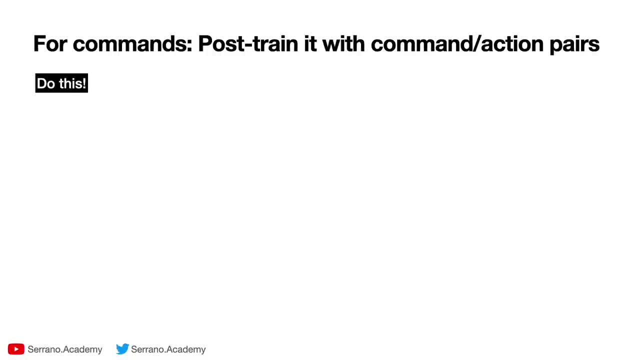 Another thing you should fine train the models for is for commands. So, for example, if you say: do the following thing, then the model must do it. For example, you can tell it to write a poem about elephants, or to correct your code, or to write code that does a particular thing to write. 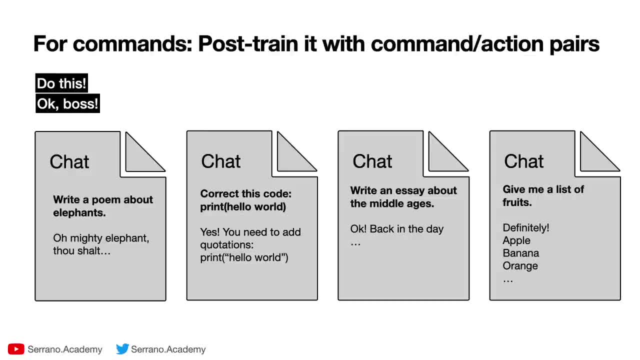 a particular essay about something, or to simply give you lists of things, etc. etc. So you need to build big data sets with commands and then the command being executed in order for the model to learn that when it's given a command, it has to follow it. And, as you can imagine, there are a lot of other use cases that you 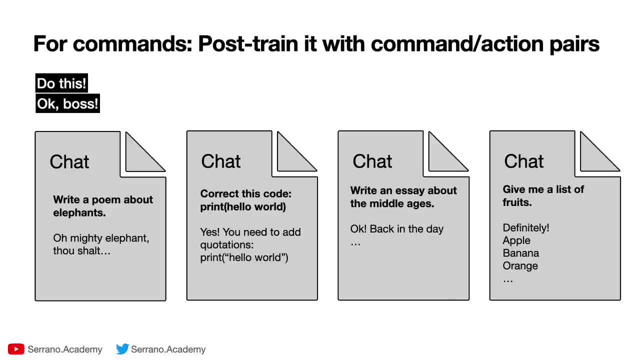 would need to fine tune your model. So I'd love for you to actually think of other cases where you would have to fine tune a model for it to work well, And feel free to put them in the comments. It would be lovely to have a discussion about it. 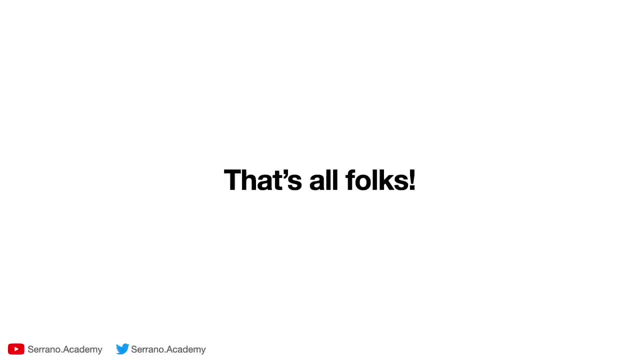 Alright, that's all about transformers. Thank you very much for your attention with this video, which was a little long, but we went through the whole thing, Just like the previous two videos. this would have not happened if not for my friends Joao Jay and Omar. 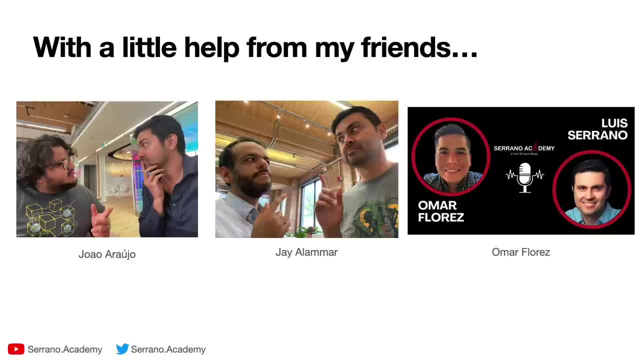 who actually explain transformers to me in much detail. In particular, there's a podcast I have with Omar that I've linked down in the comments. It's in Spanish, but if you speak Spanish I think you will like it. And if you like this content, we have a lot more at LLM University by 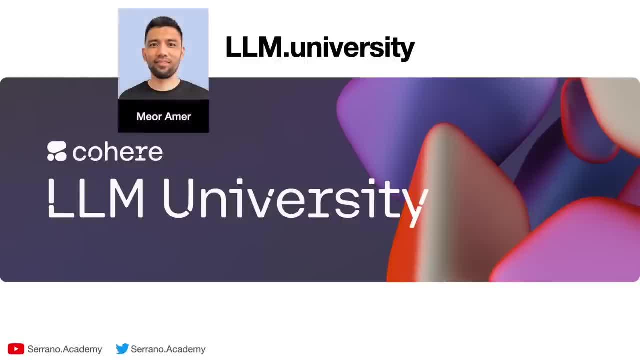 Cohere that I've built with my two colleagues, Mior and again Jay. This is a comprehensive course on transformers and the, where we have a lot about large language models, including introduction and a very conceptual explanation followed by a bunch of labs on many, many topics, including prompt engineering search. 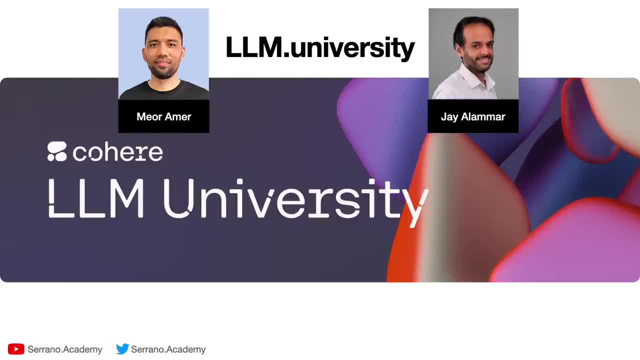 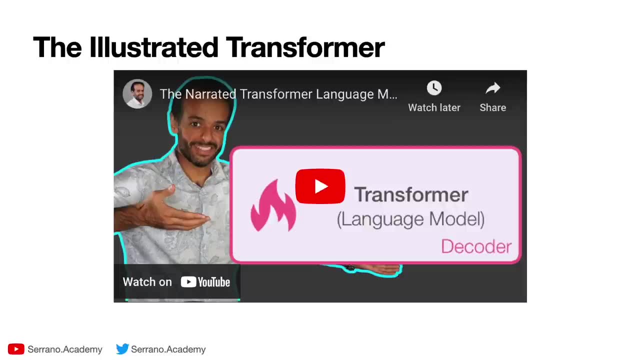 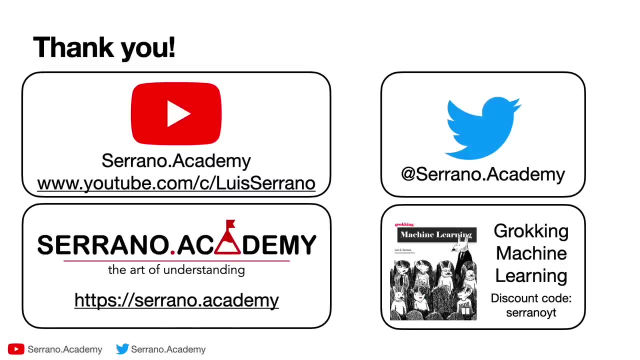 deployment and much more. and, in particular, if you want to go for more details on transformers, i recommend the illustrator transformer, again by jay, which is a really, really good video and blog post. this is where i learned what the transformers are, so thank you very much. here is some information. 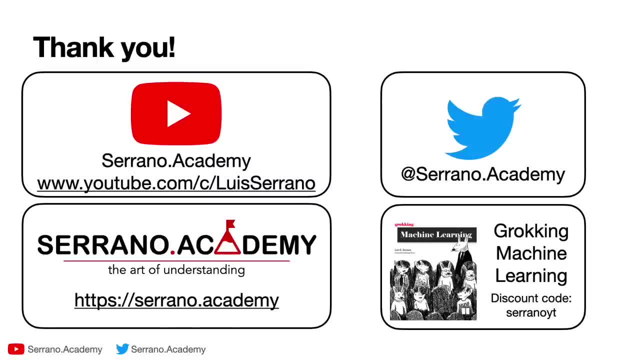 if you like this video, please subscribe to my channel- it's serranoacademy- and hit like and add a comment and share with your friends. i love reading the comments that you leave, in particular when you leave good topics about future videos. many times i've made a video about it because 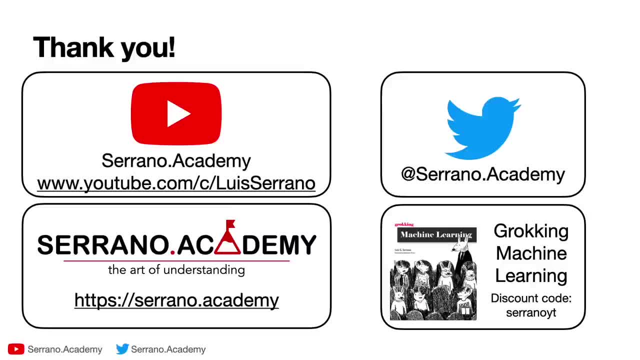 it gives me good ideas. you can also tweet at me serranoacademy, or check out my page, serranoacademy, where i have all these videos and also a bunch of blog posts, and i'll see you in the next video. bye and code and different things, and i also have the book rocking machine learning, which i